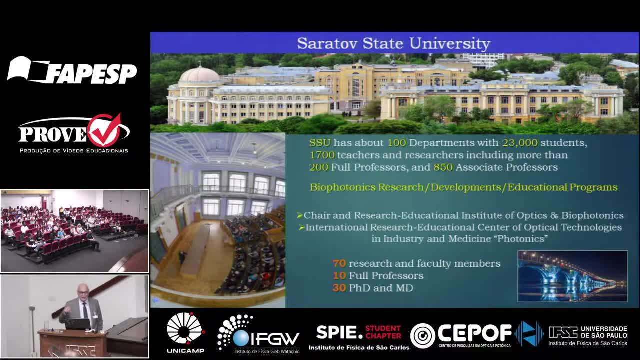 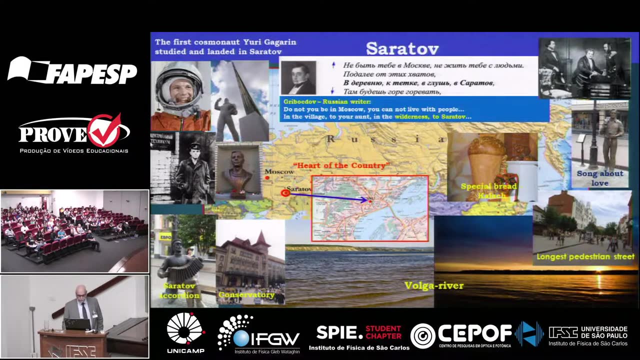 And also, as we discussed yesterday with Kristina, your city is a student city as well. Saratov is also a student city. So a few words about Saratov. what for we are famous. Indeed, the first astronaut was studying in Saratov. 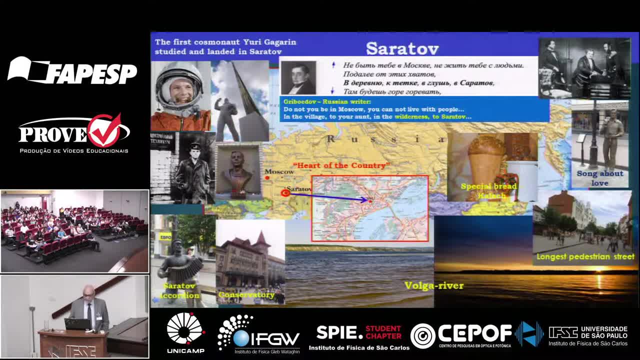 and also he landing in Saratov. so this is. we are proud about that. His name is Yuri Gagarin, you have to know. Also, we have some other famous for our country, maybe all over the world, things like Saratov Accordion, for example, the first conservatory in Russia. 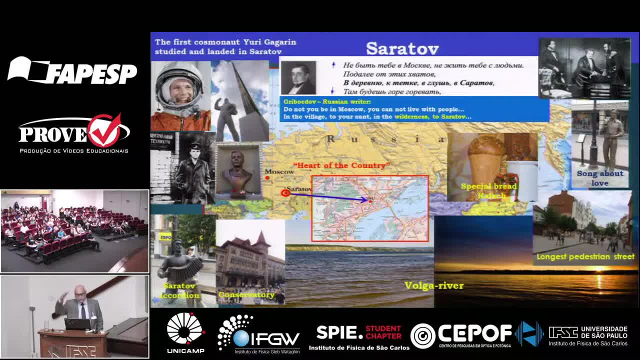 and also some special bread like Kalach, very big one, and song about love and long pedestrian street. so we are welcome to Saratov And also our meeting also. indeed, Volga River, it was not maybe so big as Amazon, but rather big river as well. 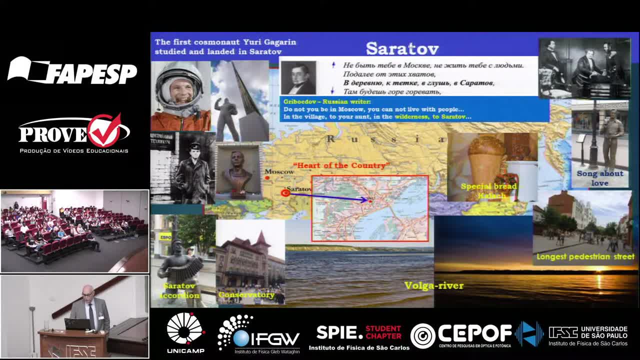 So also some poets also used our Saratov. maybe not very good for us, because Gribayedov said in his one of poems that he is sending her daughter not to live in Moscow but go to Saratov to wildness. 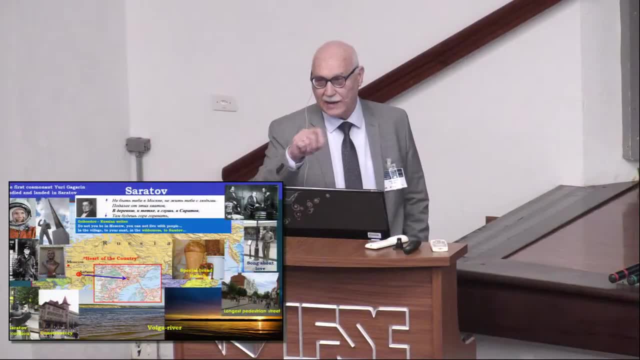 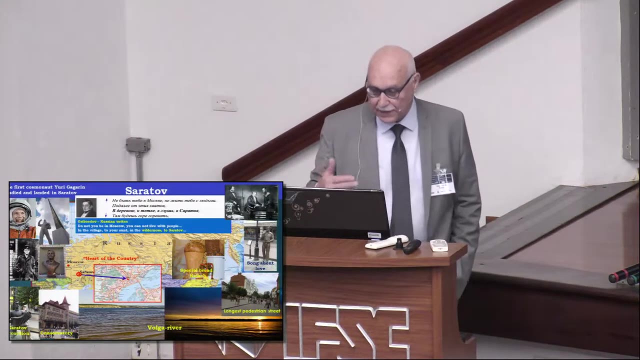 But when I try to understand what wildness mean in English or in Russian, he used another word which can be translated not like a wildness, but heart of the country. So and we are consider ourselves as a heart of the country indeed. 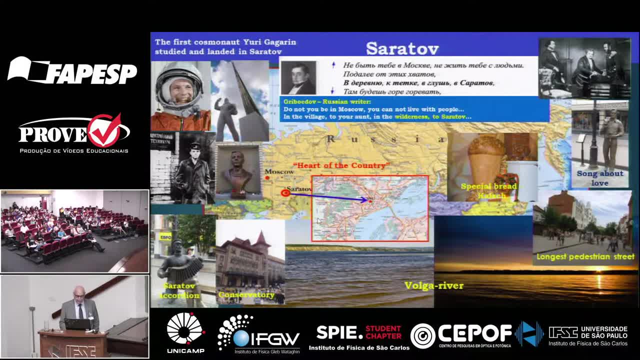 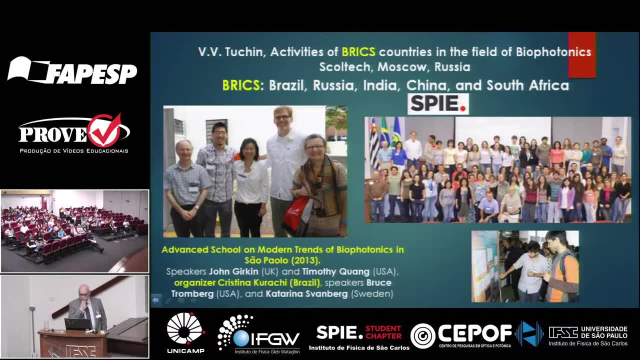 So our university is not far from the bank of the Volga River and you are welcome to visit us. So another good thing that I maybe one year ago I was invited to make a presentation on biophotonics of BRICS countries. 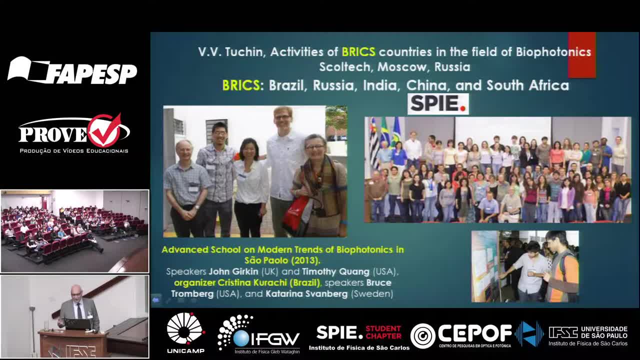 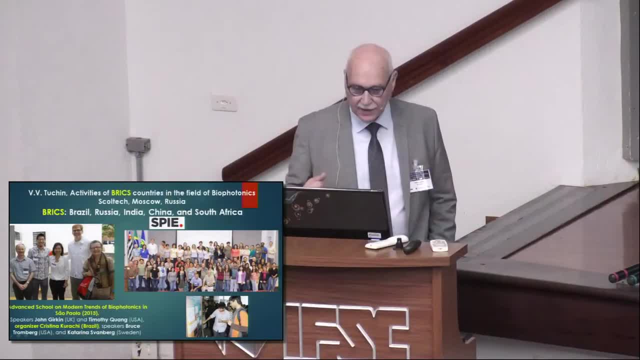 So you know that Brazil, Russia, India, China and South Africa- we have a joint economy cooperation, like BRICS countries, And I was invited to talk about biophotonics in these countries. And when I look for the activities, 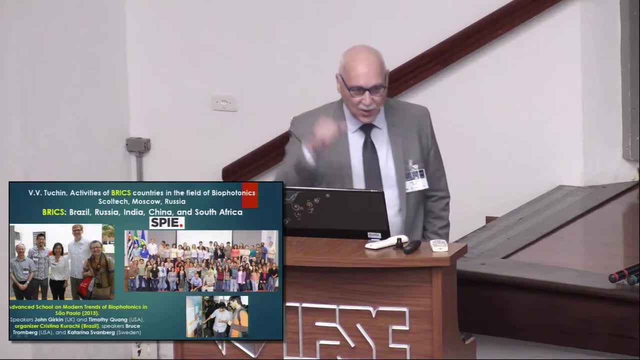 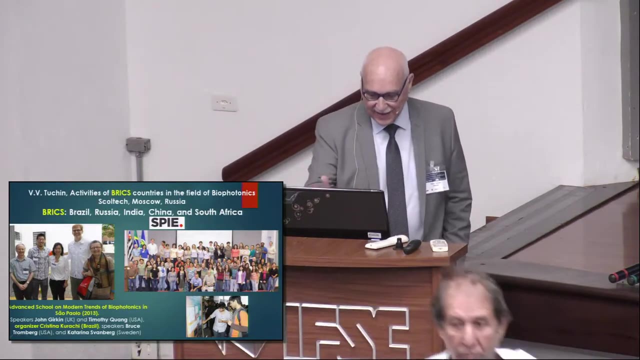 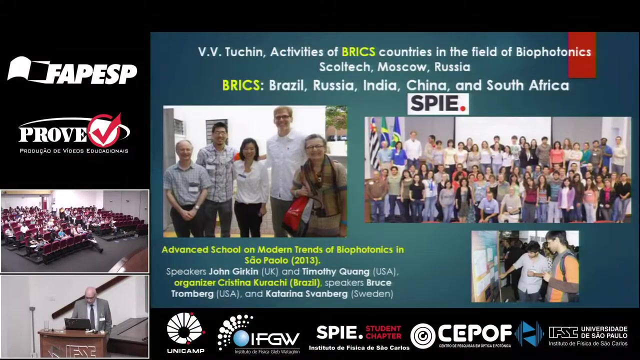 indeed, I knew about activities for a longer time in Brazil, And so I found this school. You see here Kristina's picture, And also among this I found at least four of them are my good friends, including Bruce Romberg, Katarina Swanberg and others. 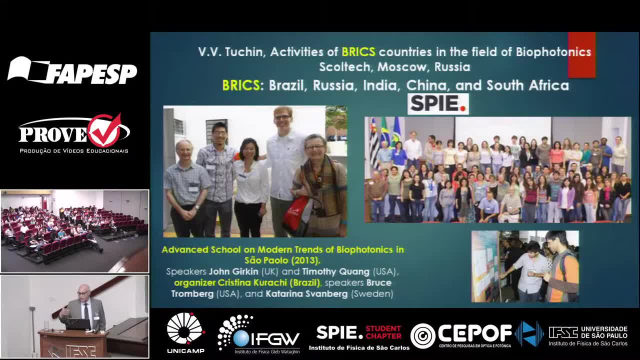 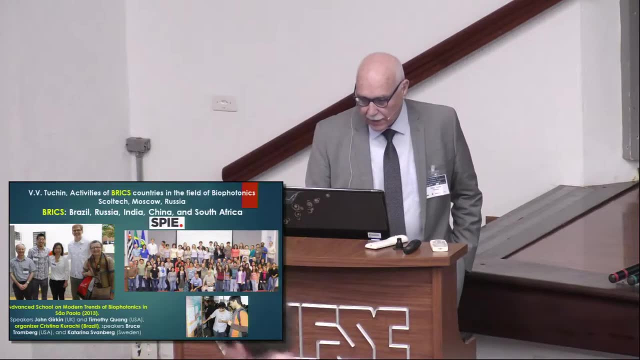 So, and fortunately, in a couple of months I got invitations to this school, So I was very pleased. It's some kind of communication which are independent of us. So therefore I'm here and I'm very happy. 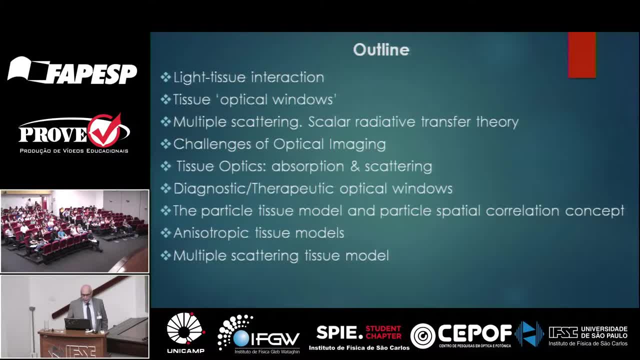 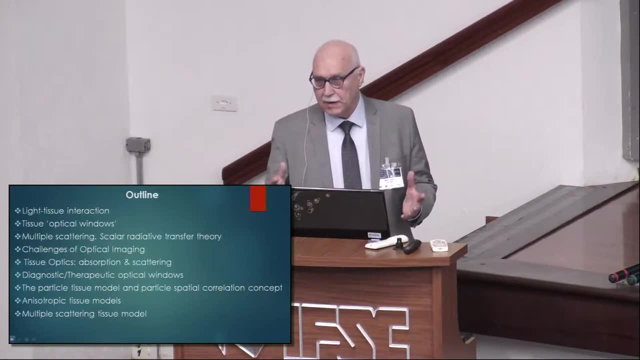 This is the outline of our of my lecture today. I would like to remind some maybe basic or fundamentals of the tissue objects And if you will have some question, please ask. or if I will be too fast, please stop me and ask question, and so on. 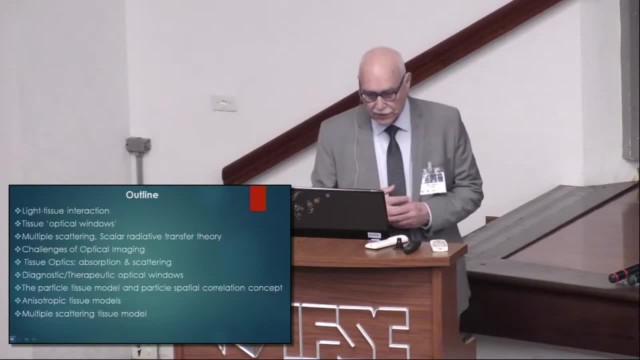 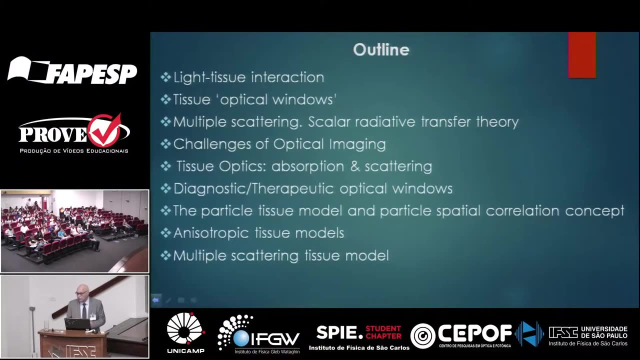 But today it will be some fundamental, so basic research or basic results. So we will discuss problem about tissue optical windows because it's very hot And yesterday night we discussed this because fortunately also two different groups. 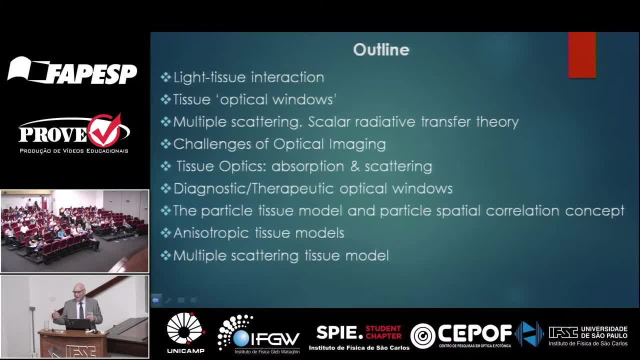 group of Alfano- Robert Alfano, who recently pay attention to the broad range of the tissue windows, And the Brazil group also helping him to worked out this problem, And independently we did it in our group also because, due to many new lasers, 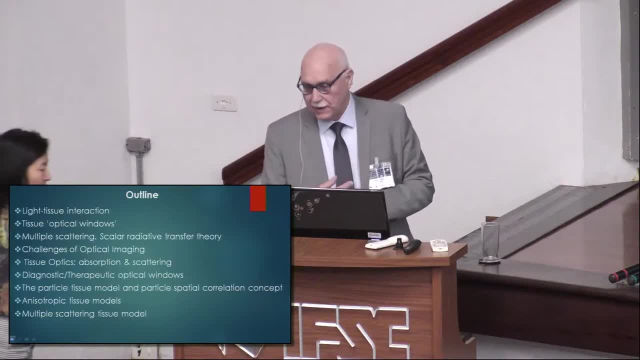 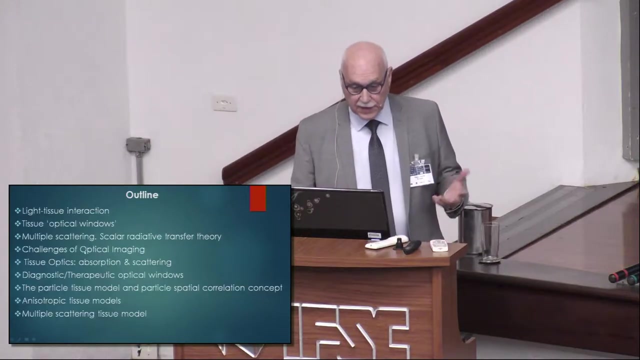 it is more and more interesting to open or to find or describe these windows for broad, very broad wavelength range. So indeed we will discuss multiple scattering, but not so in depth. So I only show you because it's. 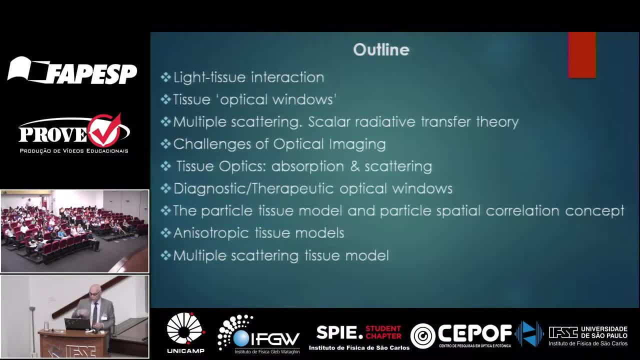 I need a lot of time to describe it totally and then we'll recommend you some books at the end of my lectures. So some discussion about the problems with optical imaging, you know, and some basics, as I said, about absorption, scattering. 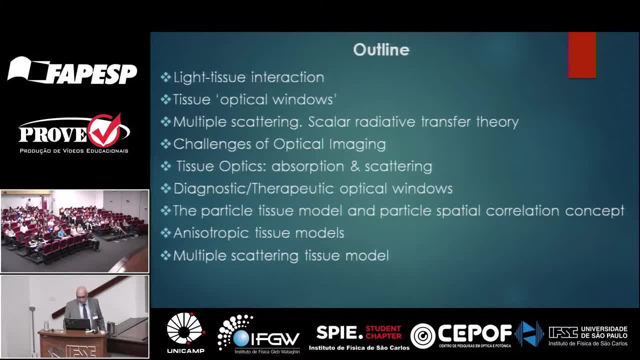 and anisotropy of scattering, And also we will maybe concentrate it today on the particle tissue model and particle-spatial correlation concept. Unfortunately it is not well discussed in literature. So because we have two approaches, One of the multiple scattering, 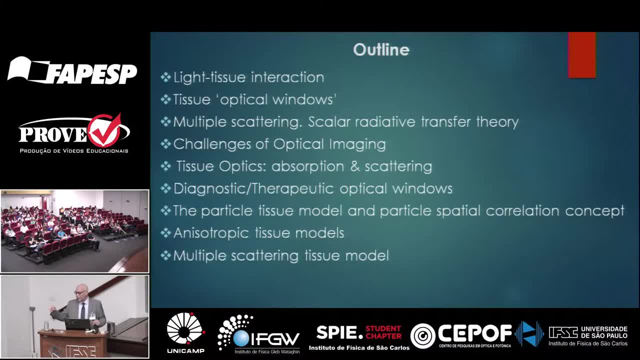 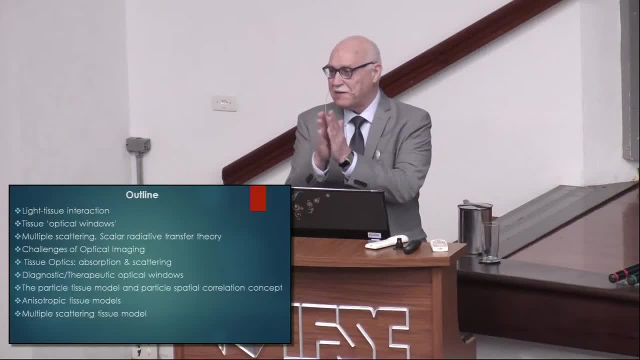 this is radiation transfer theory, Another one like Popescu, Professor Popescu, describing very thin layers of tissue with some diffraction on these particles or scatterers, And therefore, but our dream is to join both these approaches and to describe as fully as possible. 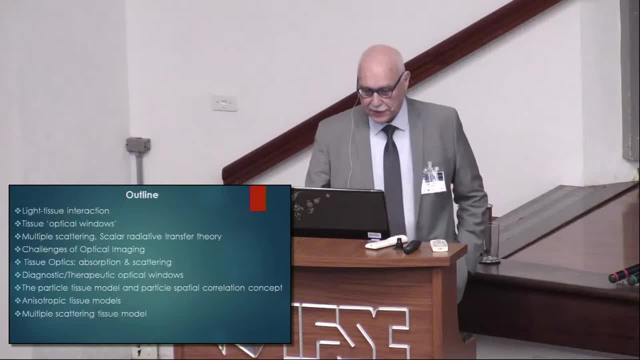 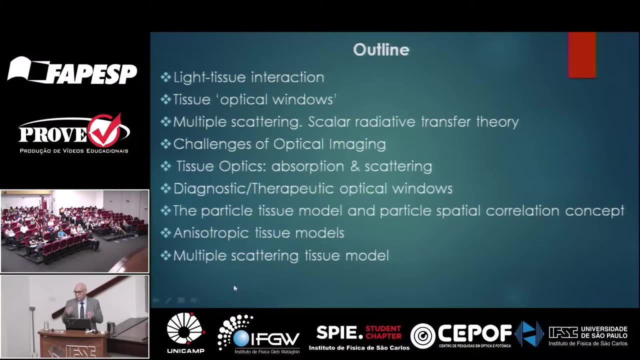 the light interaction with the scattering media. So then, a little bit about anisotropic tissue models, but from the point of view not scattering anisotropy- but it will be used indeed- But also due to polarization properties of tissue. 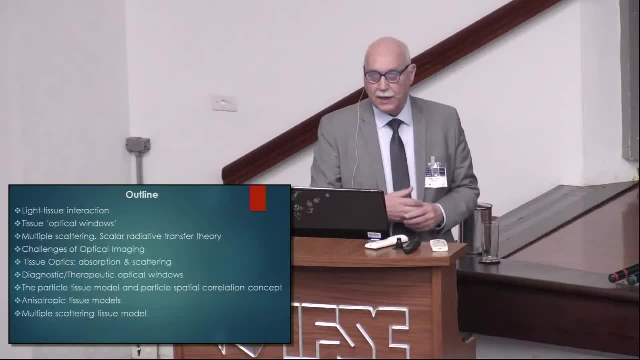 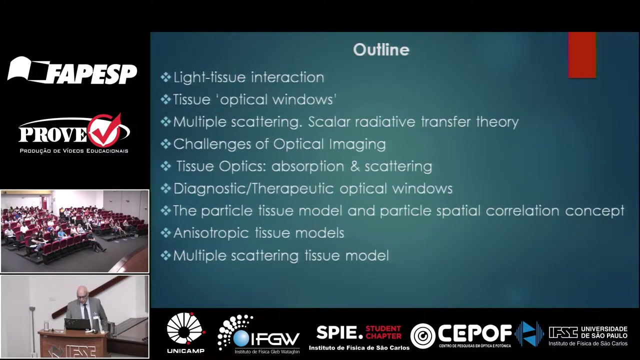 how the polarization can be transformed by these structures like tissues. And finally it will be some. I think I showed it twice, probably it's. maybe we will see. Probably it will be tonight, But you will see. 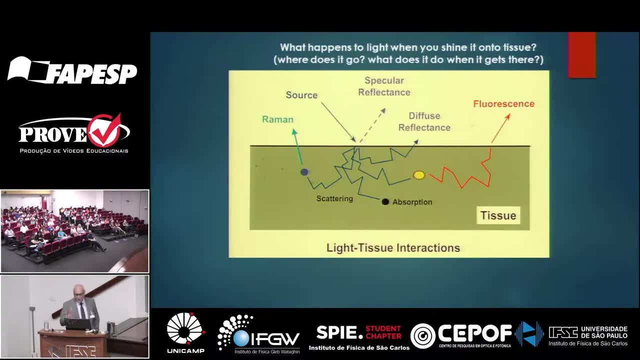 no, So it's okay. So this is, I would like to remind this is very famous maybe- picture which showing that when light source incident or light beam incident on the interface between the tissue and some ear here, by the way- 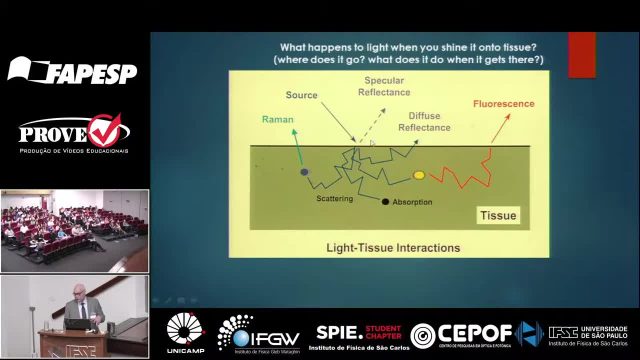 it can be not ear in real tissues, it can be water, for example, like a stomach and something else for endoscopy. And you have, indeed you have to have, some specular reflectance. specular reflection due to reflective index of the tissues. 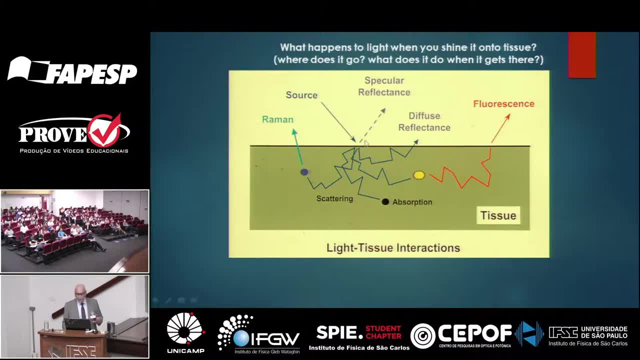 about 1.4,. for example, You have some for ear. you have 4% here which is immediately reflected. It's easy can be measured. Then we have some scattering events. They show, showed here, like this one. 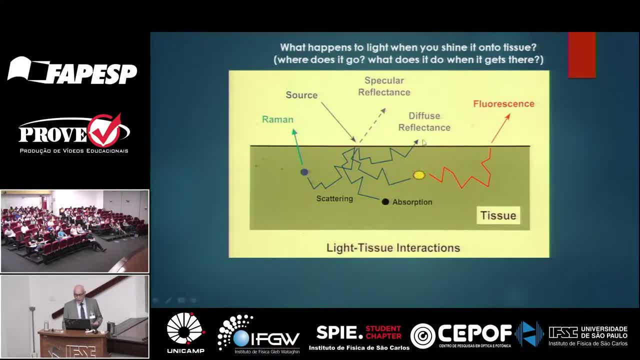 And this beam is so-called diffusion reflectance, which are very smooth and for any direction you can find some intensity. So this is so diffusion, part of this reflected signal. So indeed, if we have some multiple scattering, many events of scattering, 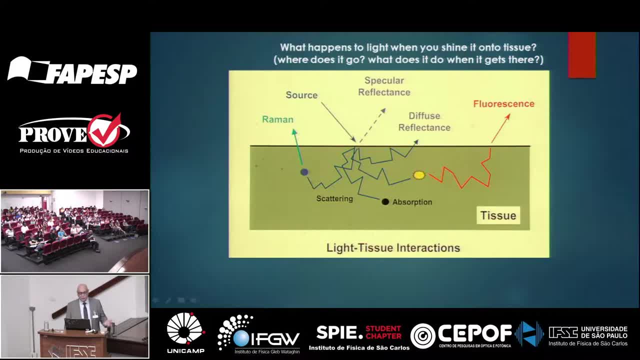 finally, we have some absorption, So energy transform to the heat and we can heat our tissue. Indeed, for many tissues in the visible light. we have quite different absorption coefficient and scattering coefficient. One hundred times more scattering than absorption. Therefore, 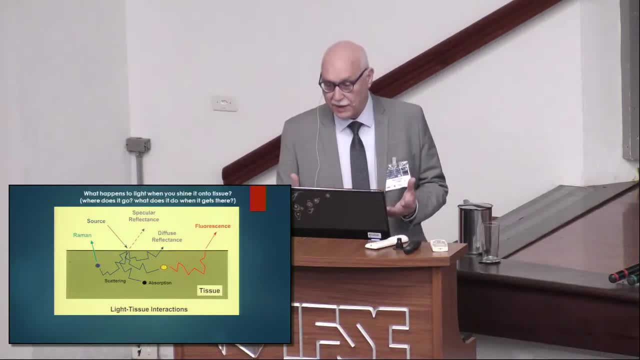 the probability to be absorbed is very rare, But still, if light traveling everywhere, finally it will be absorbed. And besides absorption, we can induce some fluorescence If we have fluorophores which are well-fit to the incident wavelength. 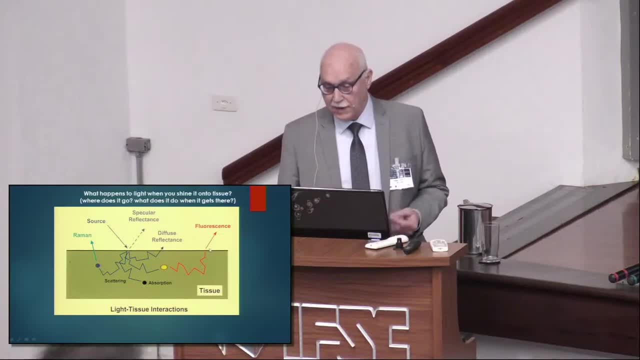 and therefore have fluorescence, which is very productive imaging modality. you can use endogenous chromophores or exogenous ones. So, and for the Zynec therapy you first found, have to found these cells, cancer cells. You stain. 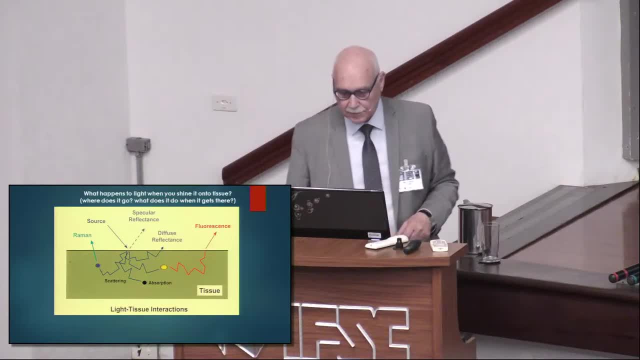 your cells, and then you can kill these cells, And this is some kind of photodynamic imaging and photodynamic therapy, Or now it's Theranostics, Because both modalities in one one technology. So indeed we can provide not only elastic scattering, 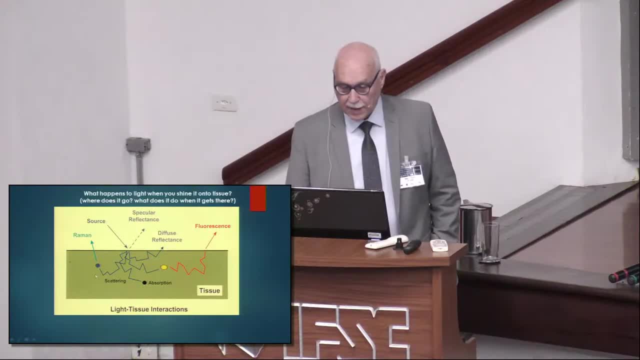 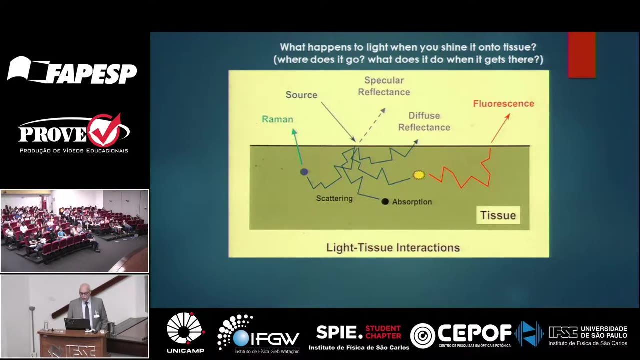 as it's shown here, but also some inelastic scattering which can be detected as a Raman signal. Also very, very powerful instrumentation and technology to characterize tissues and cells on the molecular level. So only one light beam allows you to have a plenty. 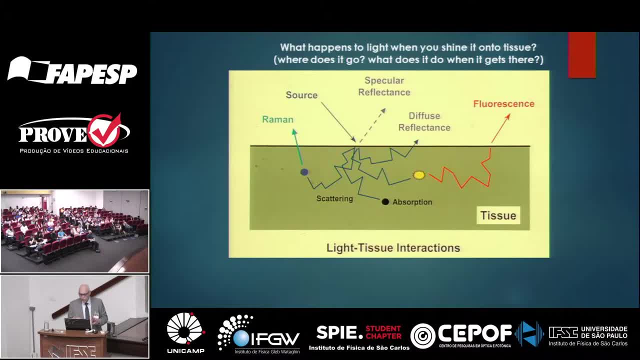 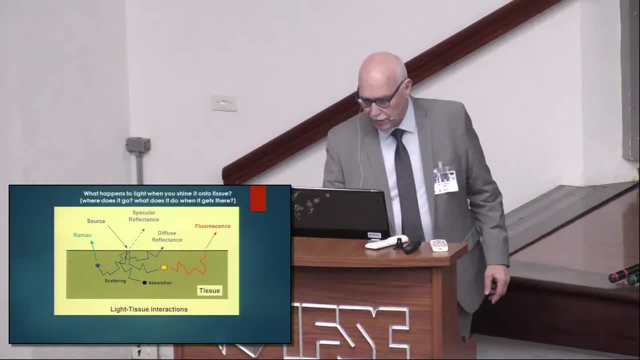 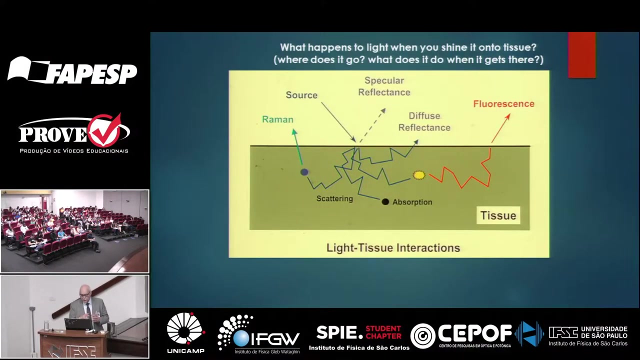 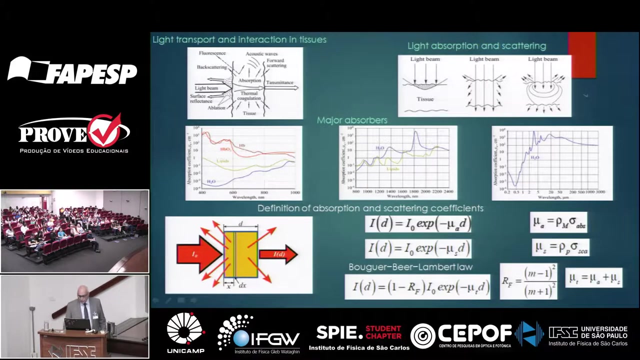 of different approaches to quantify parameters of the tissue And to get valuable information about the tissue from the point of view of molecular structures and also from the point of view of some structures, of the scatterous structures of the tissue itself. So also would like to 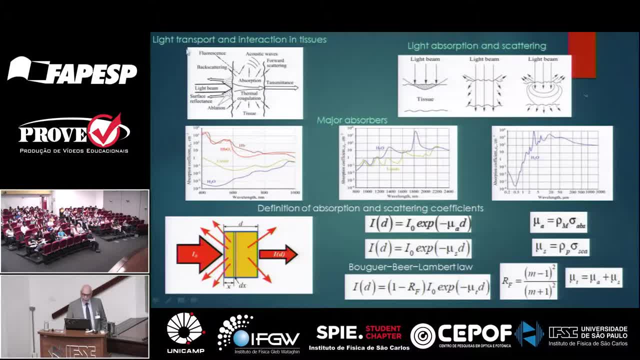 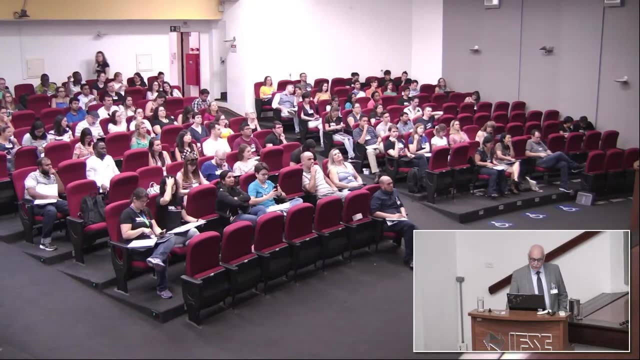 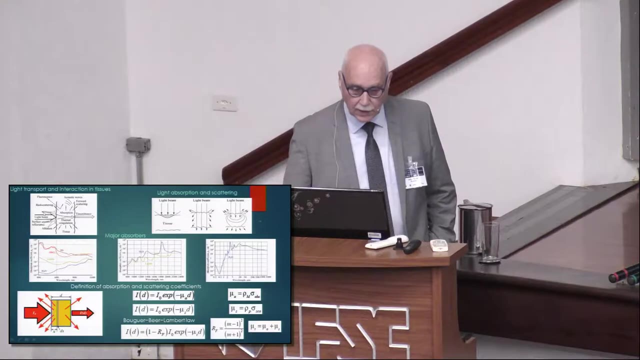 to show here what is in light transport and interaction of tissues. You can see here that light beam, this is a piece of tissue which can be absorbed and also attenuated. Then if intensity rather big we can provide some, some ablation here. 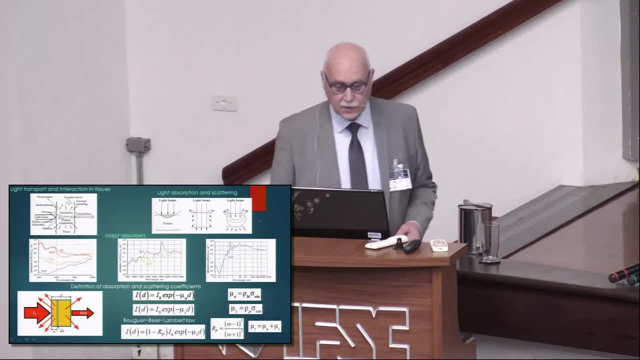 if the penetration depth is not very high into tissue. Also, if we can change the wavelength and also to provide an elevate energy and that in that case we can provide here some thermal calculation, and also from the point of view of imaging we can use forward scattering. 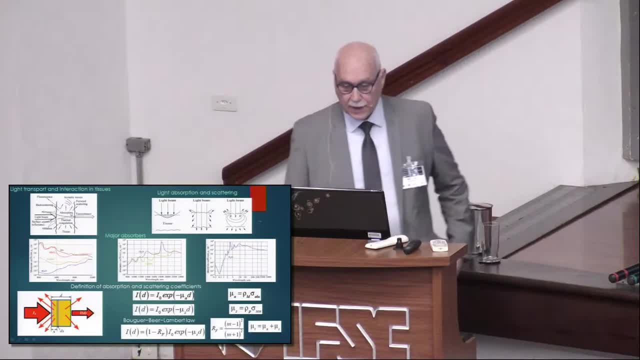 back scattering, fluorescence and also acoustic waves as well. So on the right you can see what is scattering and absorption. To the left we have absorption high. So no low penetration depth. This is light beam, this is tissue and it is. 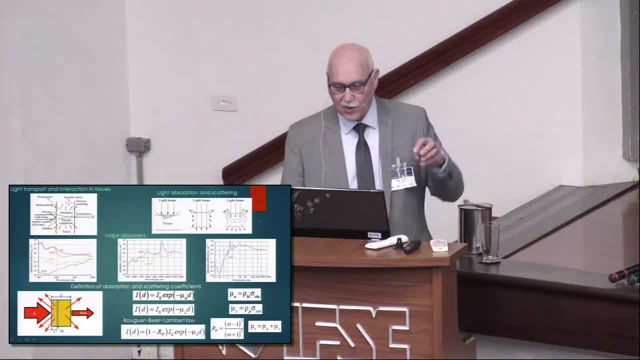 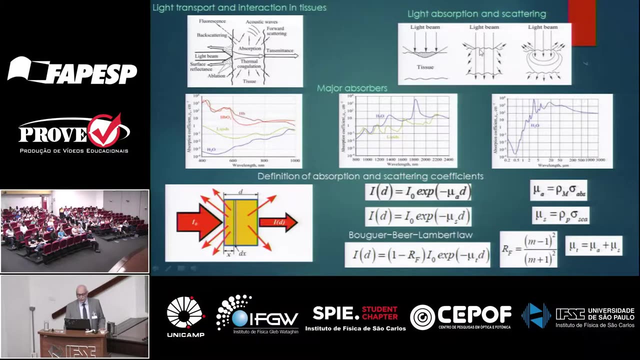 good to have some ablation, because all energy concentrated on this superficially and you can layer by layer ablate your tissue. So another point: when you have some low scattering- sorry, low absorption, and therefore scattering also can be here high, but absorption is much higher. 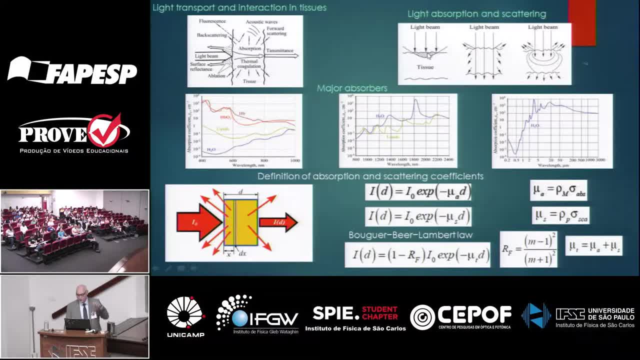 and therefore it doesn't work, and so you have ablate immediately, and in that case you have a low absorption and the same tissue with low absorption can show you a collimated beam or ballistic photons here and some scattering. So that depends only if you can. 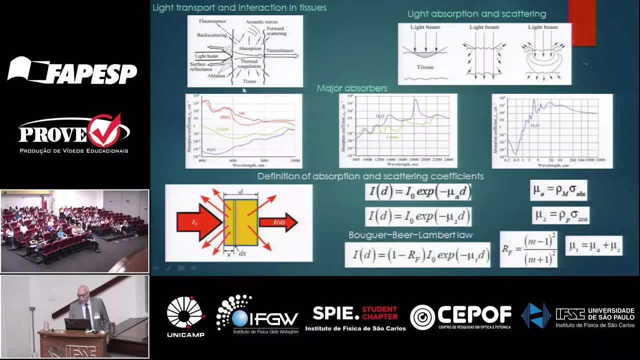 change wavelength of your beam, for example. And another situation when you have absorption and scattering more or less comparable. in that case you have a diffusion not really comparable, but more or less indeed. So you have. you allow to be low absorption, allow beam to diffuse. 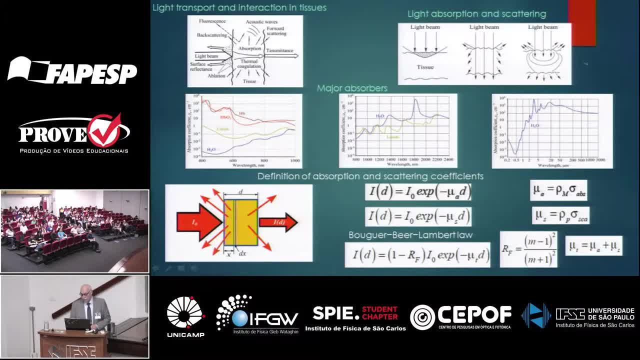 around And so it can be used for diagnostics and some therapy, because sometimes for photodynamic therapy you need some shining, or for for photoacoustic therapy, photoacoustic imaging, you have some shining of big volume of the, of the tissue. So also, you see. 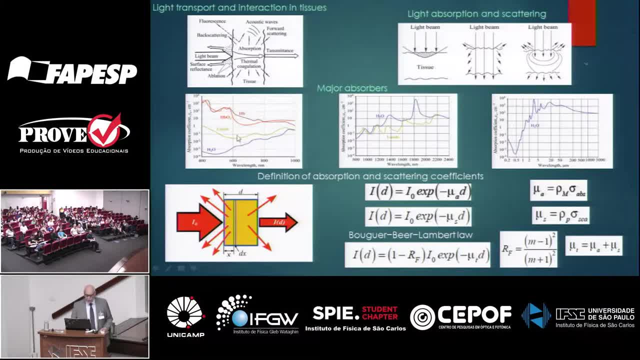 here some absorption spectra of force like hemoglobin, oxygenated hemoglobin, lipids and water. Water, you know, the main component of the soft tissue, about up to 90%, for example, for cartilage and normally it's 75 for soft tissue. So 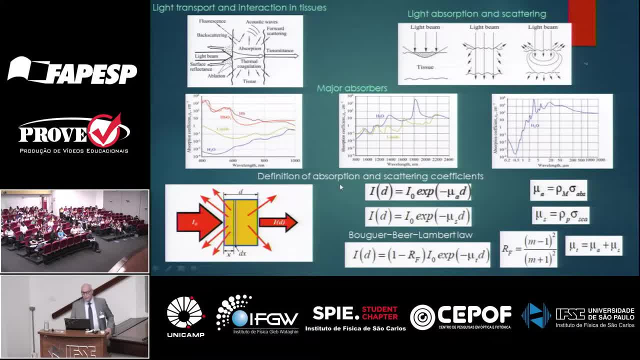 this right you see more detailed spectra of the water and lipids in the in the in the approximation of the single scattering. you can use Bugers-Beers-Lambert law in this form, where this is intensity, incident intensity and this is detected intensity which are transmitted. 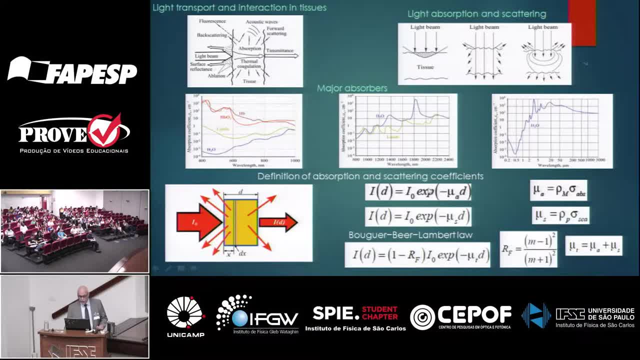 from this layer and you can. this is well known exponential dependence. and if your media is is totally absorption absorptive, you can measure absorption coefficient, which is depends on the density of the particles and scattering absorption cross-section, and the same for the scattering, purely scattering, media. if 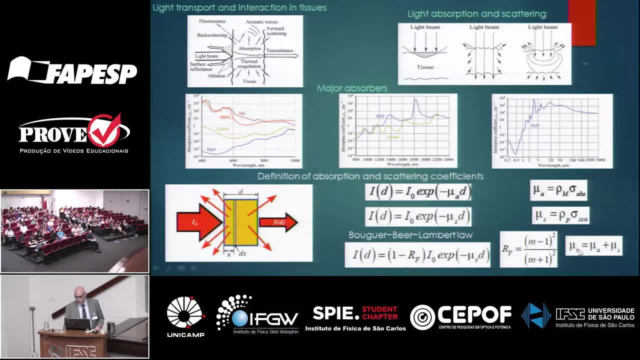 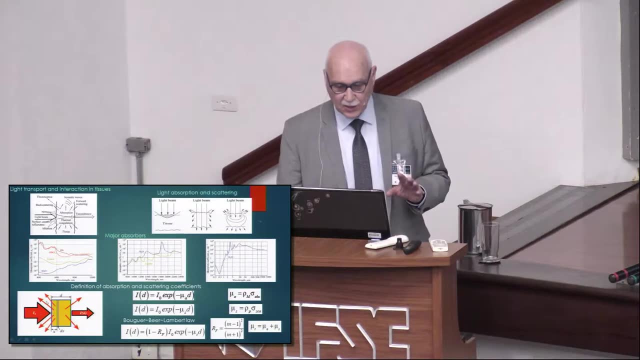 you can introduce attenuation coefficient or extinction coefficient, which is some of these two scattering and absorption coefficients also. we have for many, especially for the mid-infrared. we need to account for this specular reflectivity because this is reflective of the surrounding media, of the tissue and surrounding. 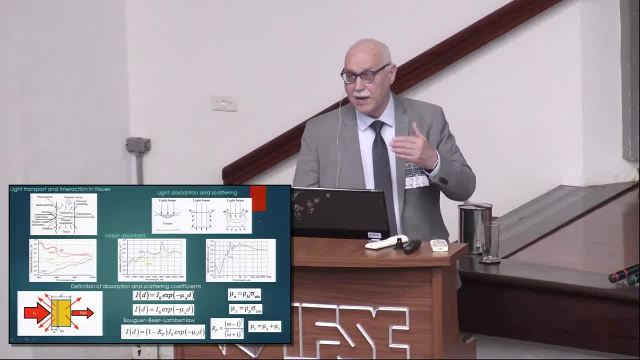 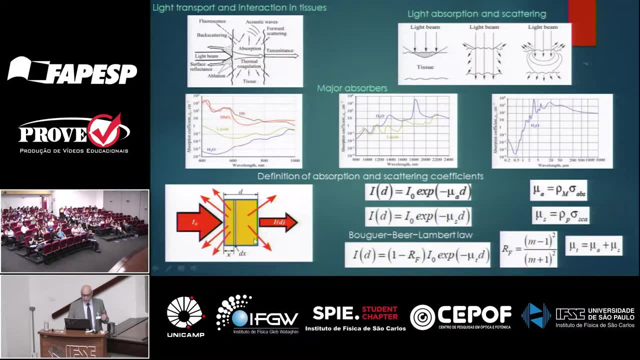 media and therefore this coefficient for the mid-infrared should be high. so about maybe about 30% of incident light can be reflected back immediately- not scattering, but immediately on this interface, like this fully written booger bears lambert law, including the attenuation for both scattering. 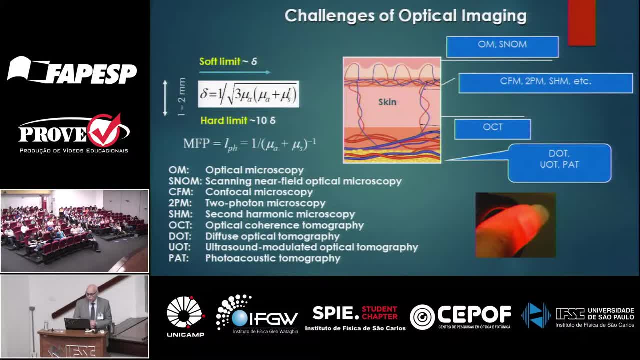 and absorption media and specular reflectivity. so what is the problems with the optical imaging we can see here, that we can see using the ordinary microscopy only some superficial layers, only cells on this, like stratum corneum here, because example of skin is shown here we can. 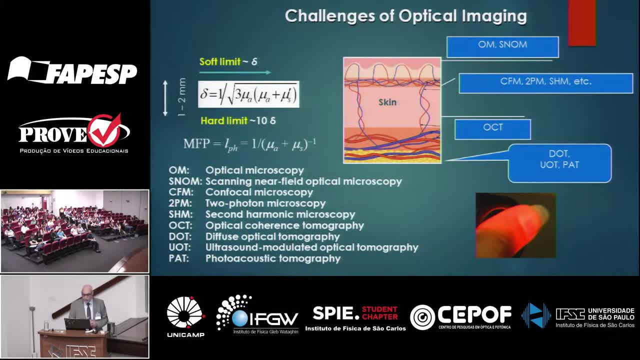 see that the beam is 1 mm small and the structure is quite small and not well visible. you can see that it is quite large. so it Forward, and I would like to show here the penetration depth first, but then we will describe the equation from which we can. 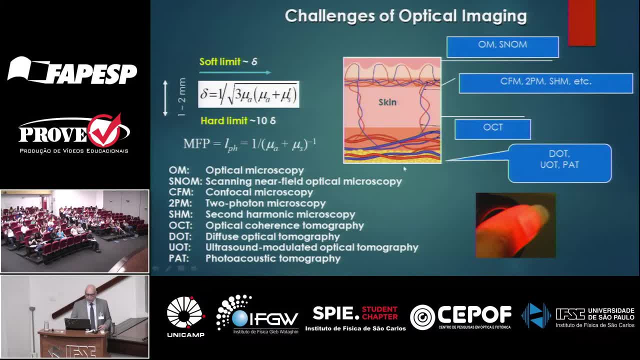 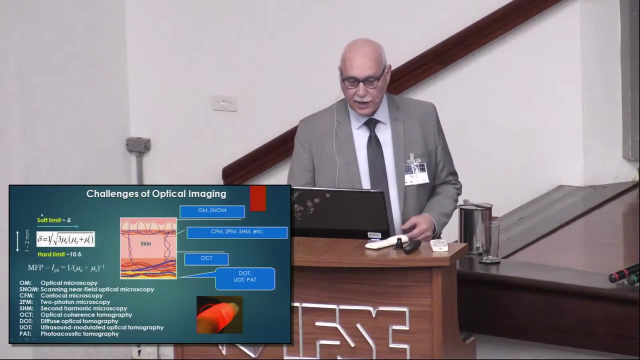 Express or deliver this Formula. this formula Received in the Diffusion approximation when they have a multiple scattering, a high multiple scattering, and It show us that the penetration depth of the light, where the light beam attenuated in e times or 2.7 times it is not high attenuation. indeed, we can work for. 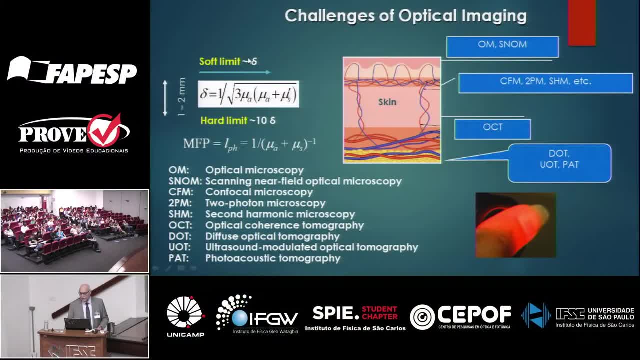 So-called soft limit when a light attenuated only 2.7 times and also up to 10 Delta, it's because we can detect single photons here, when they relate here. so this is not maybe for modern instrumentation. it was not strict Limitation, but still we have to. 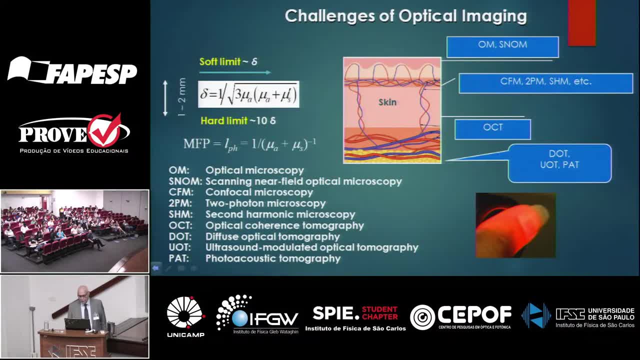 to have something on this big distances. so and we see here that indeed absorption is very important, but the so-called reduce scattering coefficient is which is 10 or up to 100 time bigger than absorption coefficient. you can- this is the K point and you can control due to wavelengths. 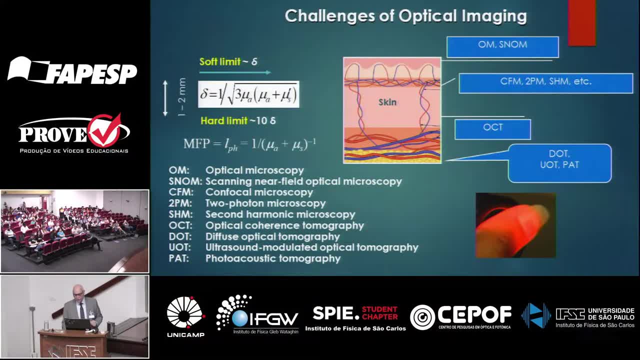 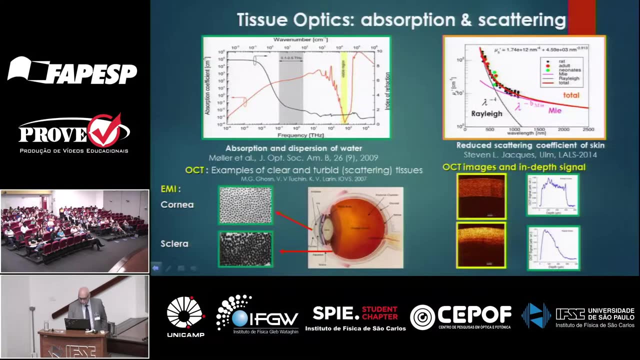 go to infrared, for example, or using optical clearing to reduce scattering, and you can improve this penetration depth in very wide range. so so, once again, more detailed spectrum and we are interested in the very wide, very broad wavelength range. this is here the wavelength range and the visual part on this yellow and 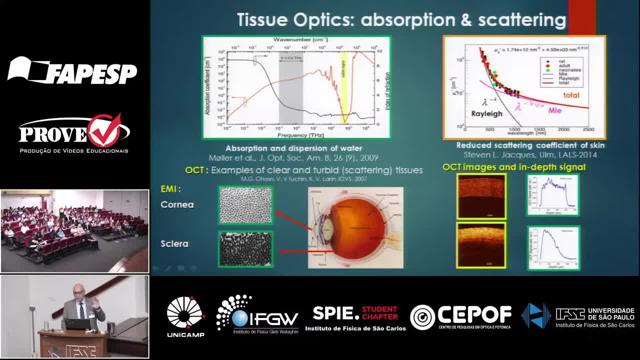 this is for water and, as we know, for soft tissue, water is the main chromophore. therefore it's a good model of any tissue, only soft tissue so- and you see here that this is the absorption of water- can be changed maybe 1 million times from. 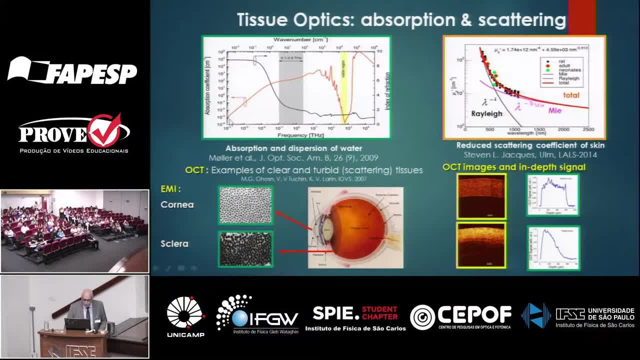 that depends on the wavelength, and for visible light we have about 10 minus 3 inverse centimeters, and for terahertz range, for example- which also of interest now- it's 10 plus 200 inverse centimeters, so very big range. so no penetration here and good penetration here. so about scattering: reduce scattering. 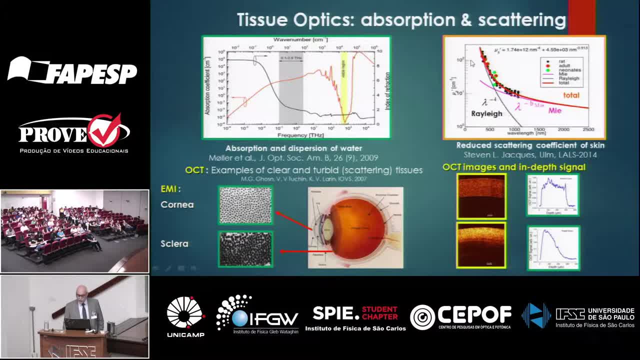 coefficient is changes also from for the blue light, for example, green light, from 100 inverse centimeters up to maybe 10 and some units for fine, for for mid infrared, and indeed here we have a relay scattering, here we have some mixed scattering and some mixture between. so we have to take into 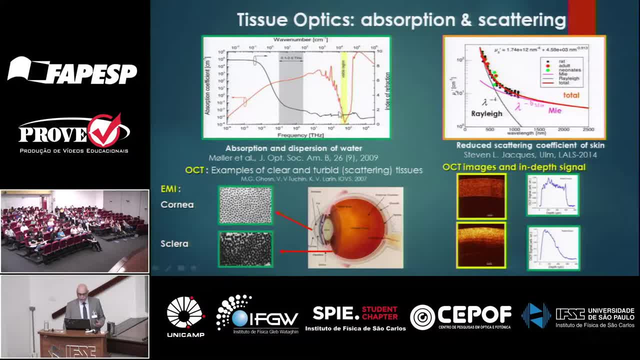 account that we can regulate in some limits as absorption, adding some endogenous, exogenous chromophores or change scattering due to optical clearing, and it may give you some benefits for long-term and long-term use of optical clearing and it may give you some benefits for long-term use. 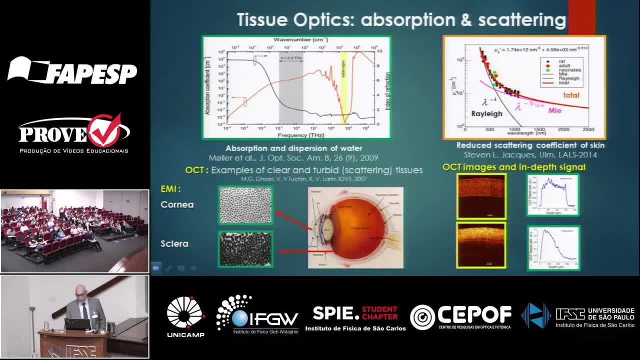 light transportation and better probing depth. also, I would like to pay attention to the two tissues. one tissue is absolutely clear, you know, cornea, eye cornea, and another, sclera, is white, so it is well penetrative. this is well scattering media, but structure the same is collagen fibers, and we will 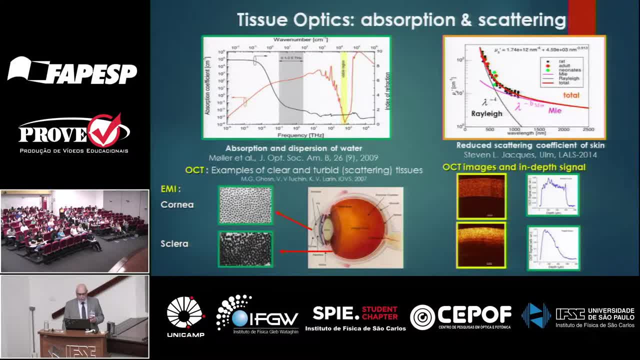 talk in details later on- and due to quasi crystal structure of the cornea, we have constructive interference when the light is transported through this cornea into the eye and distracted in this direction and therefore it's well transparent, even indeed it have to be scattering media. why? because reflective index of 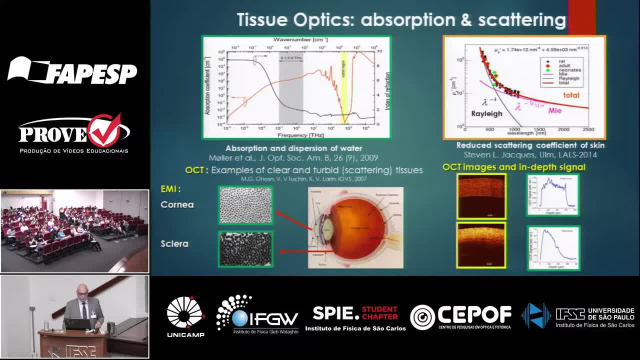 the collagen fibers is much higher than the surrounding and whispering and it is equally bright. and when it's disordered and what it is not, quasi crystal it it is white and scattered light on the different wavelengths. and another example here: optical cover. here in tomography images, OCT images for cornea and sclera, we have a pretty good reflectivity from the. 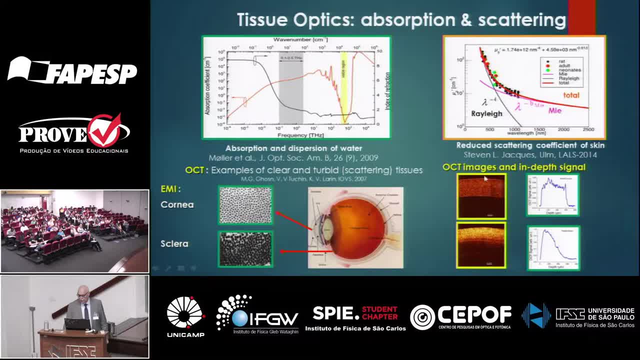 back surface from endothelial cells here, epithelial cells here, and through whole range about 0% to 20% millimeter of the thickness, and for Sclera. we have no signal behind Sclera and indeed if we try to reduce scattering we can move our system from. 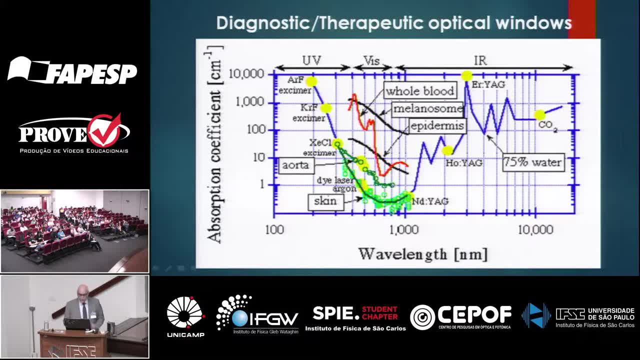 this one to this one. So this is very famous picture done maybe first by Steve Jacques- at least I found it first in his paper- and indeed this is a spectrum of the water which are good model, as I told some chromophores like whole blood. 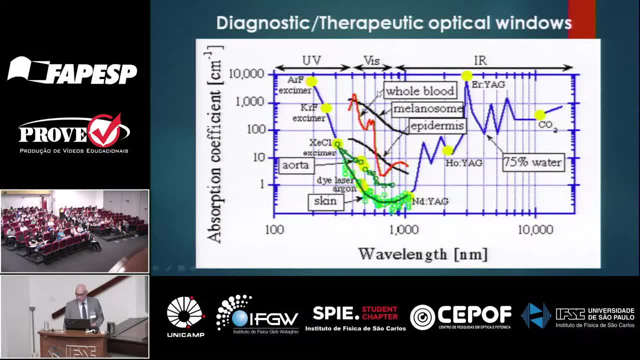 here, some, it is mostly for epidermis, for skin, and some melanin which contains in melanosomus, and also if we combine all these fractions because we have to use also for calculations of the penetration depth or absorption coefficient, different components of these tissues. indeed, we have only 5% of the blood. 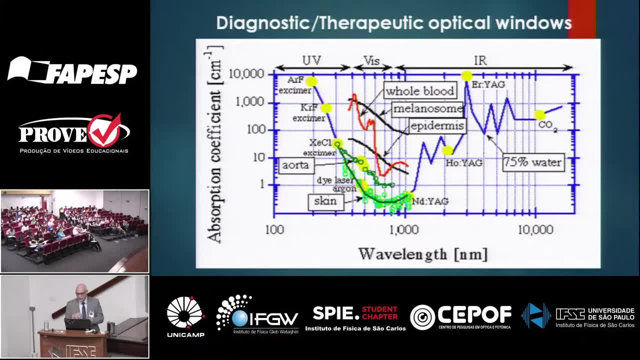 indeed we have also limited concentration of the melanin. and finally, it is interesting, you can see here that for whole skin it is very, very close to water, because indeed you can see on the background of the water some hemoglobin, oxygenated or not oxygenated, but the most if it is rather thick, rather thick, you can see that water is. 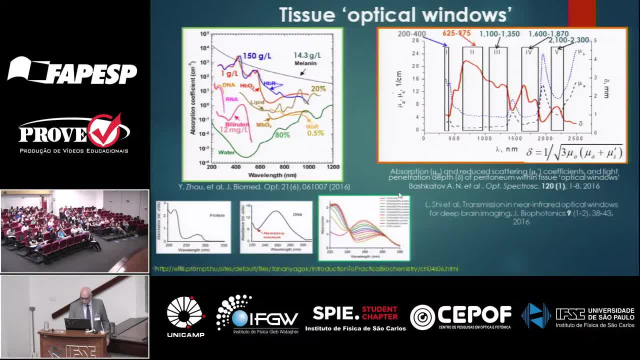 dominated here. So please look once again on the spectra now. I took this from the Li Hong Wang paper, which are recently published and well cited in Journal of biomedical optics- and please pay attention that the water chromophore- you see, the water is a chromophore- has a not very high absorption in the ultraviolet. 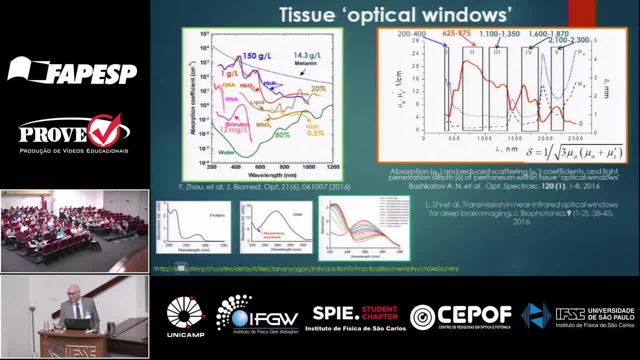 is comparable with the infrared, so that means that we have an opportunity to go in ultra violet range. indeed, if we reduce scattering, because and if we reduce scattering, We can see proteins and DNA. and you see, here they also have some windows. This is windows for these companions, and this is showing. you can find it on the Internet. 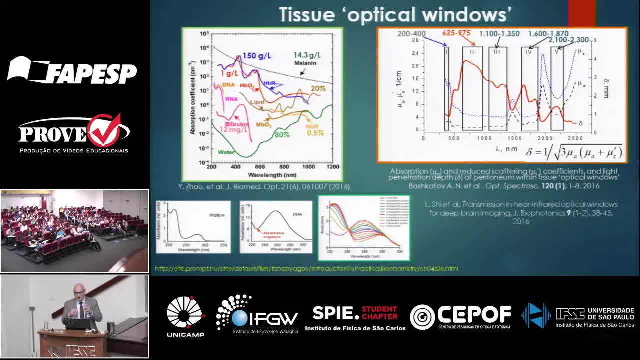 that you have a mixture of DNA and proteins, in particular cells or tissues, and if concentration is different, you can see here some kind of isobastic point here for this wavelength 240, and also I will show later on how to provide these windows. 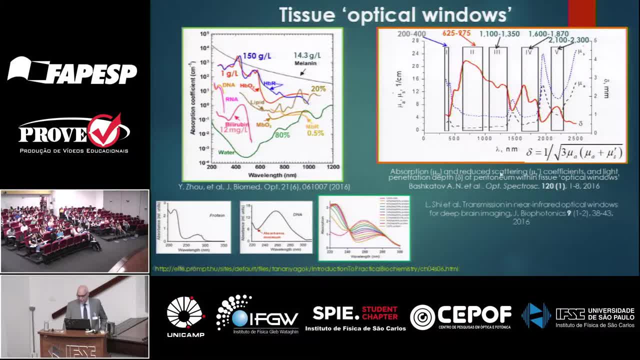 And this is related to what was done by your colleagues and together with Robert Alfana. and this is the red curve, This is the penetration depth received in the diffusion approximation, and this is the penetration depth received in the diffusion approximation. and this is the windows. this is the window which is used by everybody for a longer time. 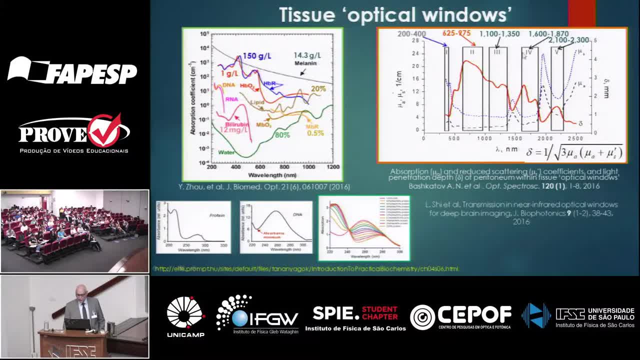 and this is a new one- windows. this is the wavelength range and I counted, not like Alfana and his colleagues, but we started from ultra-wide, so please don't miss it. and now we have the second, third, fourth and even fifth. 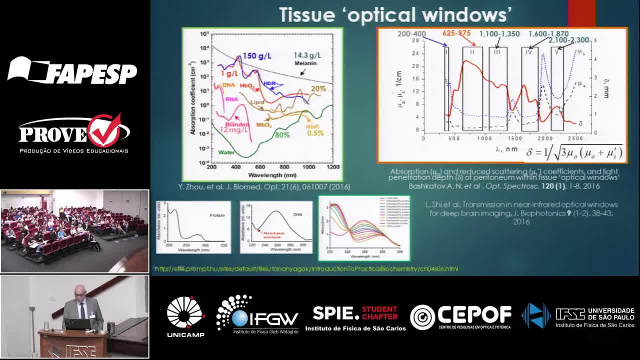 So, and the penetration depth is quite good, about one millimeter, maybe more, and up to 2.5 millimeters and so on, and this is done in particular for peritoneum tissue, and I think it's a good point to study now. 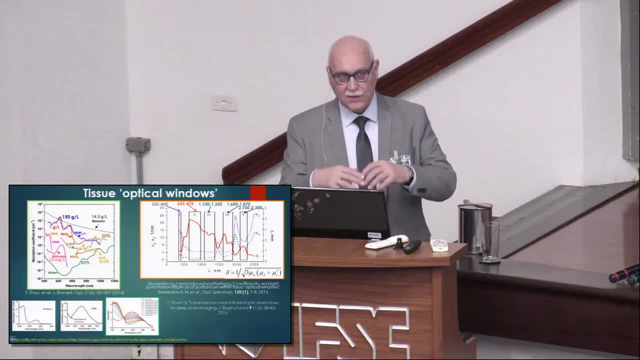 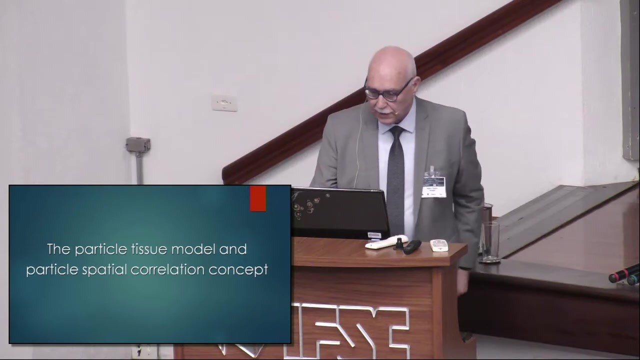 Indeed, we can. from the point of view of the optical clearing, which I will talk later on in next lectures, it is very important to regulate this penetration depth, because it depends on the absorption, and reduce scattering coefficient. So let's talk about particle tissue model and particle spatial correlation concept. 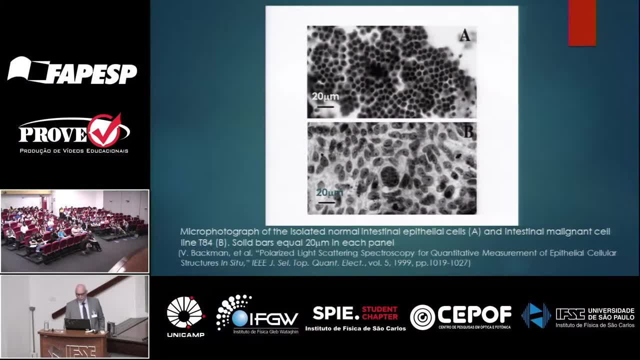 So once again very famous figure from work of Vadim Beckman and his collaborators and which show that for malignancy we have an increasing of the nuclear size and this is one of the marker of the of malignancy. 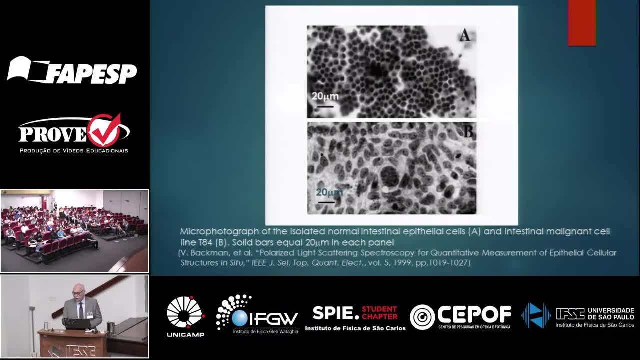 And indeed scattering is quite different for normal tissue and malignant tissue and some polarization, So we have a lot of malignancy. So once again very famous figure from work of Vadim Beckman and his and some polarization. 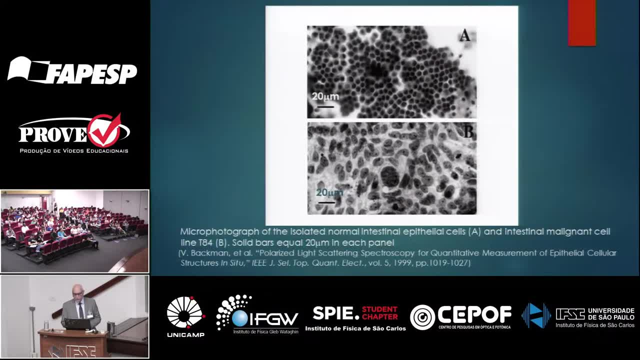 So, once again, very famous figure from work of Vadim Beckman and his properties can be changed and some intensity of scattering and so on, so on. So therefore I'm talking about that- we have to consider any tissue. 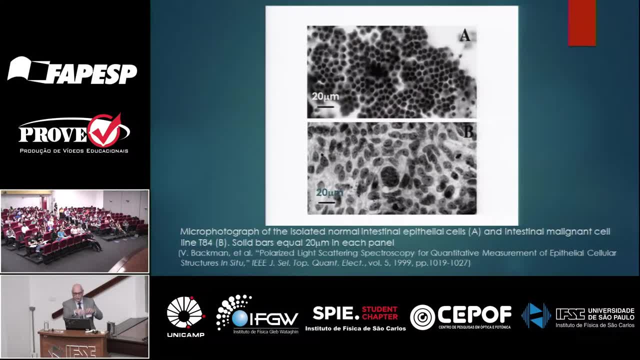 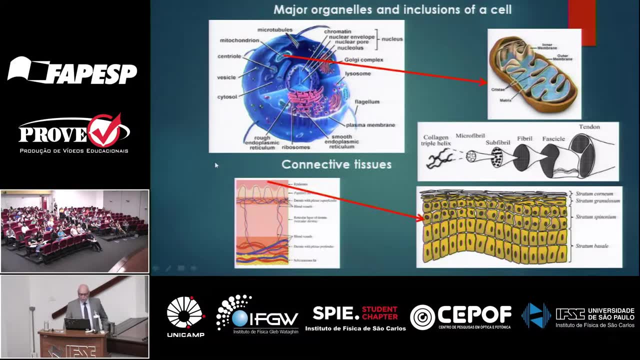 of cells from the particle point of view. We have particles with different refractive indexes, with different size. This is important Also. we can find particles anywhere in the cell. You see here nuclears, then some mitochondria, for example. 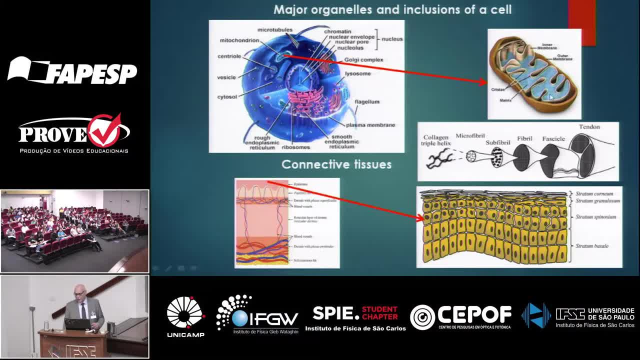 mitochondria. It is what was shown many years ago. but Britain's chance is a very good scatterer because it is miscattering. It's rather big, about 600 nanometers in this direction and about one micron in this direction, And there's also some complications here because there's 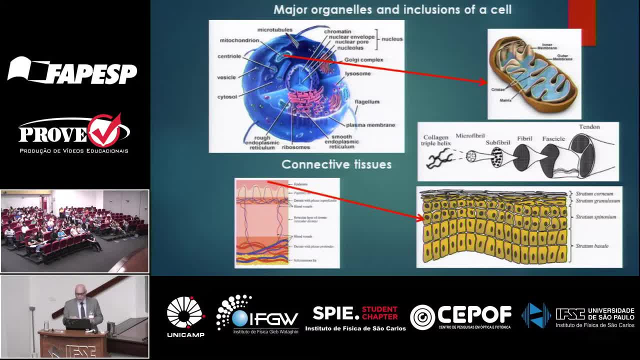 variations of the reflective index And therefore it is a good scatterer, especially tissues. here It was a special paper where, by Britain's chance, in his group, where they showed that the scattering coefficient is related to the concentration of mitochondria in particular. 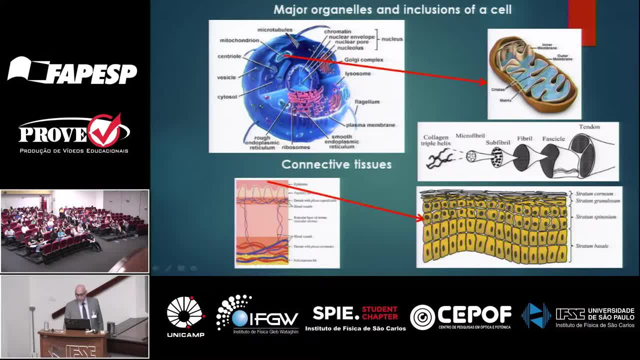 tissues. It is very important In other. if we consider some connective tissue like tendon for example, you see also very good structure of the collagen fibers, which are also particles, but not spherical particles But elongated cylinders, And so we can find any particle system in any tissue. So if we 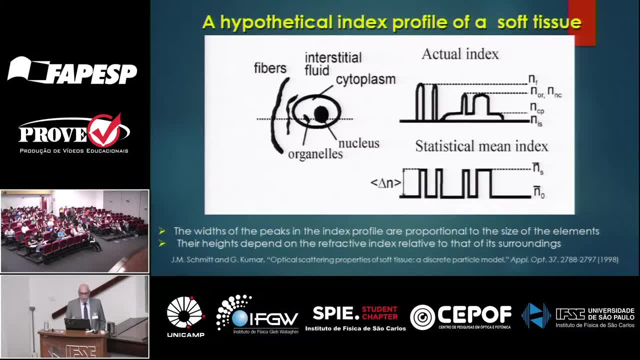 try to build some model. first of all we have to find these reflective indexes- size of the particles in order to include in theory or to make some estimation. And also- this is famous picture from the paper of Josh Mead. Josh Mead is very famous. 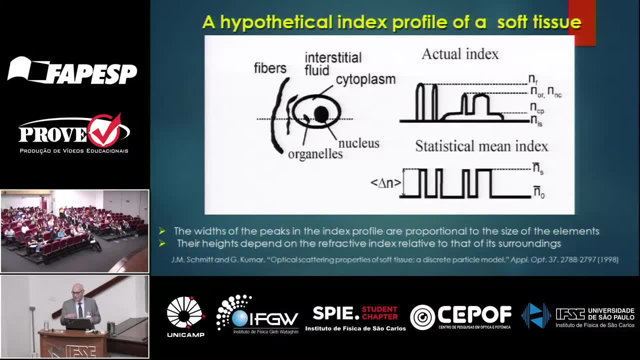 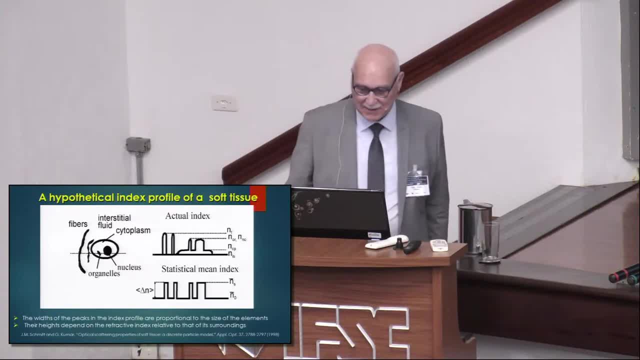 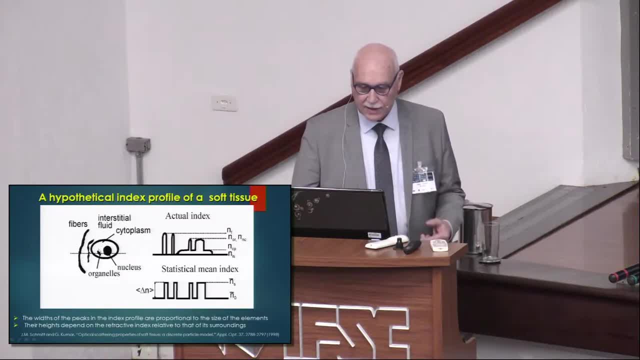 epithelial layer with the nucleus here, organelles and so on. That's typical for skin, for some mucous and any tissues. So if we will go in this direction we can see so-called actual reflective index, So reflective index of the fiber. then and here. 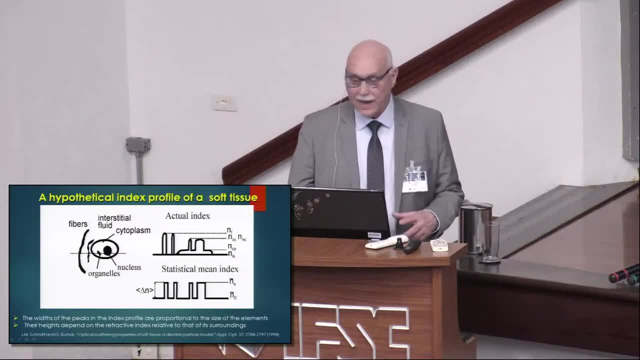 shown the thickness of the fiber, Why we are talking about thickness or size and reflective index For optics. you know this is the delay of the light, So this is optical length And we need- because you know it's a trade-off- to measure, for example, using OCT, both reflective. 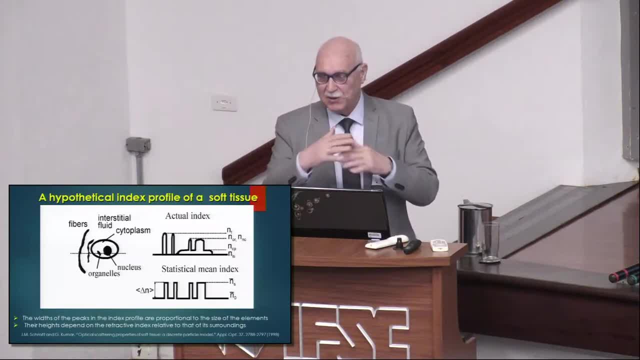 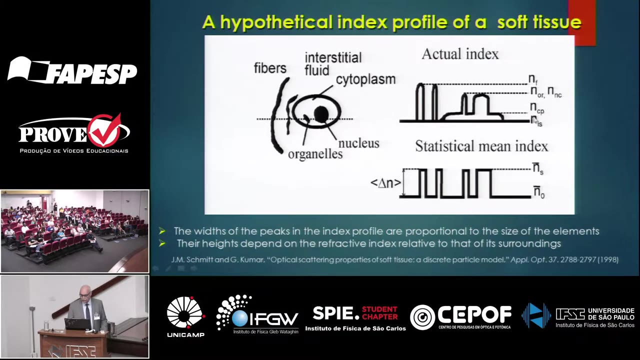 index and the thickness of tissue, And you have to find something, some different approaches to understand. So for us size and reflective index very important And indeed you have very complicated system with different one, two, three, four, five reflective indexes. 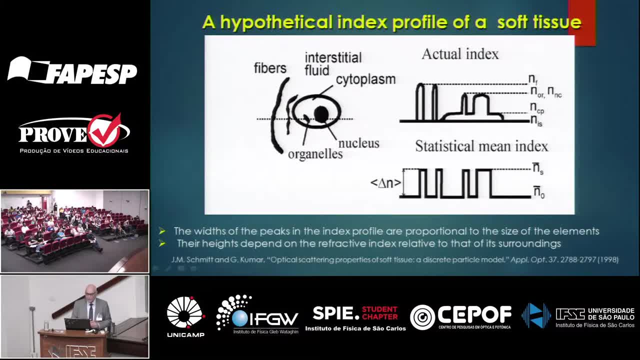 and the different size. So it's impossible to maybe to, But the people try to do it because a power of computers now is so big That you can, and many in adaptive optics, for example, And now one of the direction of the optical clearing is not to do something with the tissue, to put something on impregnate. 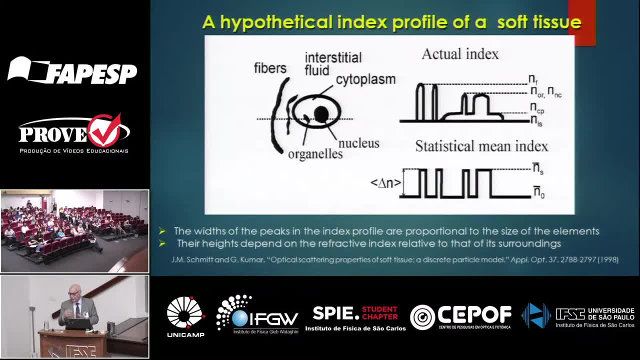 Also, you can calculate how your beam goes from the scattering, but you have to have a good model. After that you calculate all scattering events and then you can improve your beam or recognize what has happened with your beam within these turbid tissues. 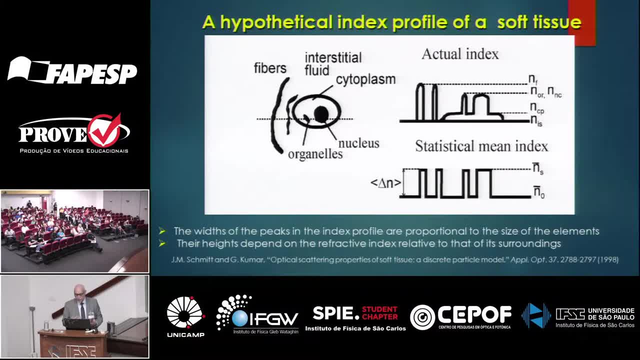 So but still to help and to impregnate by something to help to reduce scattering is much better And the combined. I would like to show you later on that combined computing and physical optical clearing is more beneficial right now. So to reduce some this system. 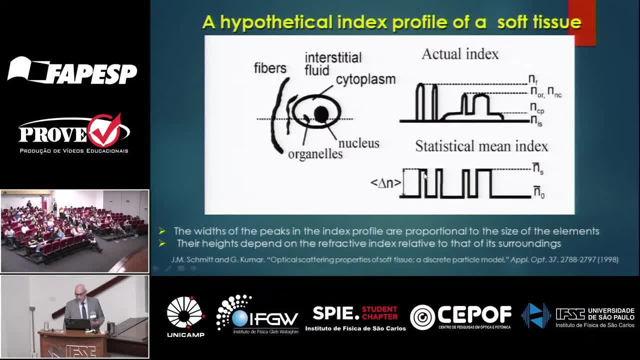 to make it more reasonable for calculations. You can find that we have two different types of the reflective indexes. For cytoplasm and for interstitial space we have more or less the same, So we can over it, And for scatterers also more or less the same. So now we have only two reflective indexes which can be. 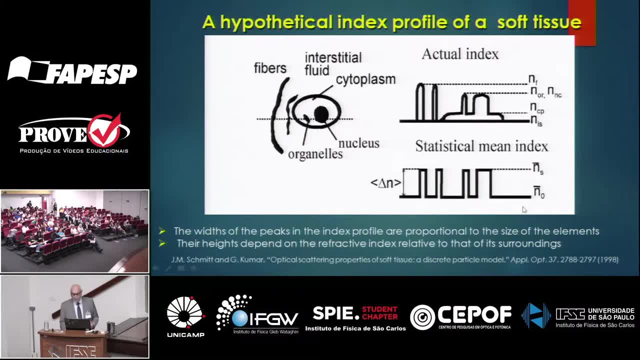 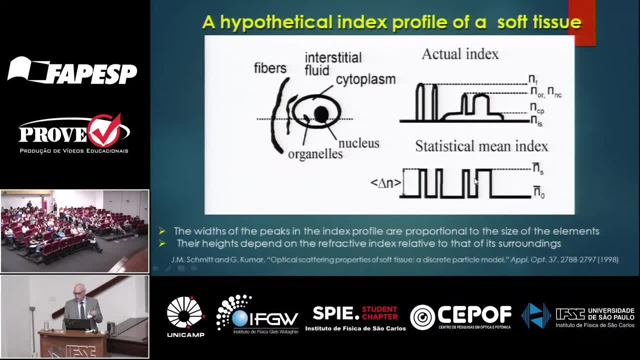 that we have two reflective indexes And you can see that we have Approximately two phased system: One big particles, one third big particles and three- two thirds of the small particles. So now we reduce our system only for two types of scatterers, With the smaller the diameters or size. with big diameters We know. 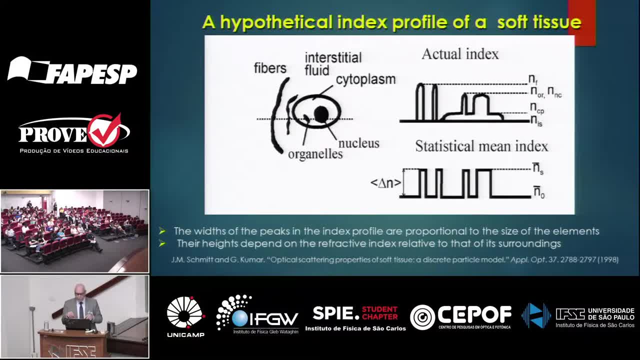 the ratio between them, and also we have the reflective indexes, particularly for eH, so I think it's something more reasonable too. and also we have the reflective indexes, particularly for eH, so I think it's something more reasonable too. وال ers expected owe. 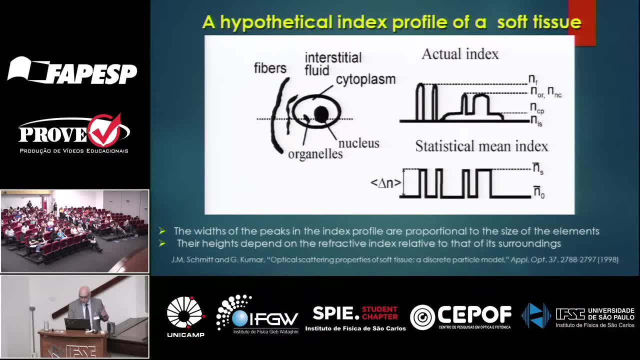 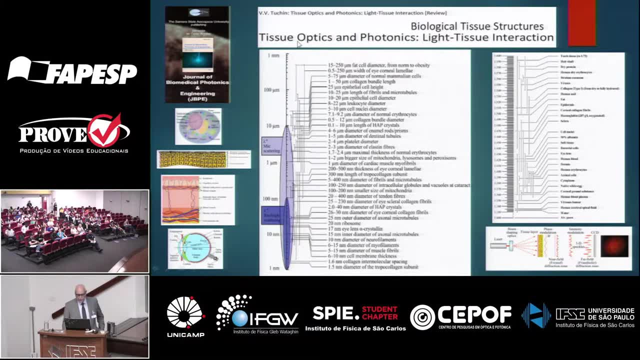 for each particle, for each kind of particle. So it is very long. You can find it in my paper: Tissue Optics and Photonics, And this is the range of the sizes which you can find in the cells and tissues. So this is, you see here, very long range. 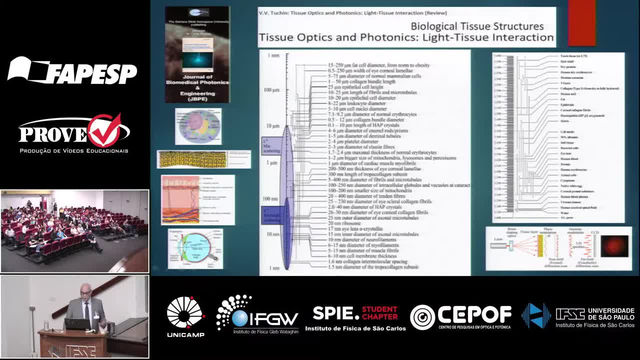 And it can be used in any calculations for estimation, whatever you like. This is size to the left And to the right. you have reflective indexes. So if you go to internet and there is a very nice site on reflective indexes of different materials, 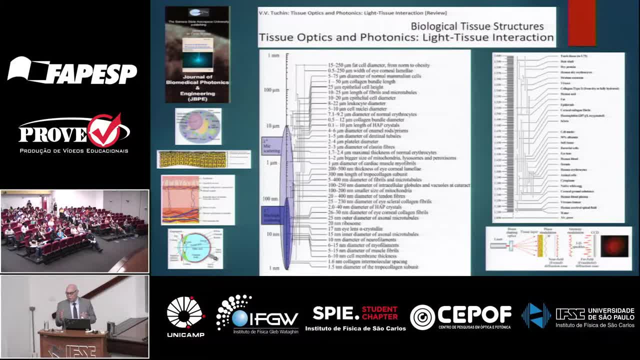 And only three, maybe four papers of results devoted to reflective indexes, measurements of the companions of tissues. So this is very important, I think very important piece of work which can be done and which should be collected to go to this database and so on. So to the right, you see here. 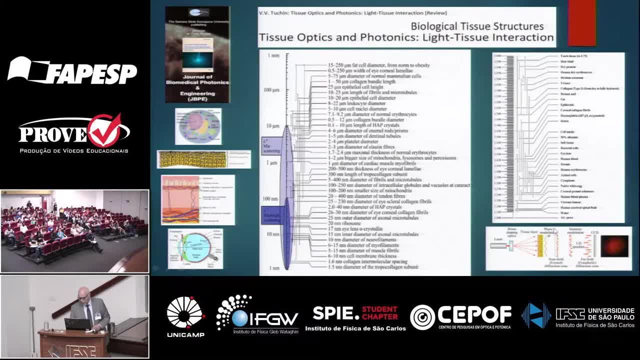 to the right here, down to the right down. you see here some speckle technology. When you have some thin layer of the tissue here, scatterers, some coherence, some phase modulation first and amplitude modulation Finally, you have a speckles. 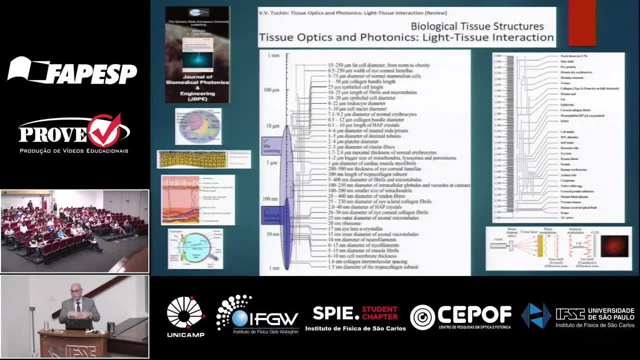 Speckles. if you have a coherent light, So we use it everywhere with this mouse, with any measure: blood flow and whatever you like. But I would like to stress your attention that the people using the speckles use it for measurements of reflective index of this media. 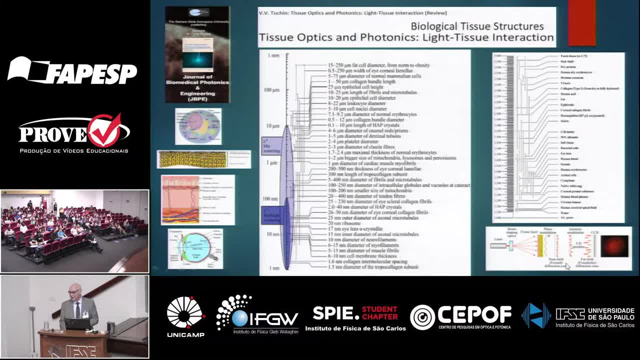 Indeed this information contained here, And this is done very recently. You can find this paper published very soon, also already published from Ziv Zalievsky from Israel. So very elegant, very simple, very easy to do. You have a bottle, you have some turbidity here, like a mill. 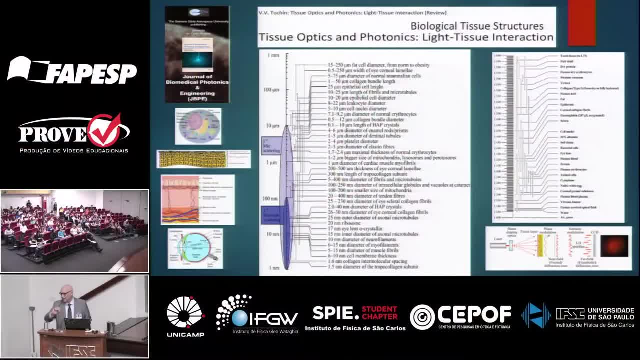 then light, then speckles, You measure a simple camera And after that you have some software to recognize. what is the change here? with the reflective index Indeed, you have model. you have to have model, but still it is well, you can test it from some bits. 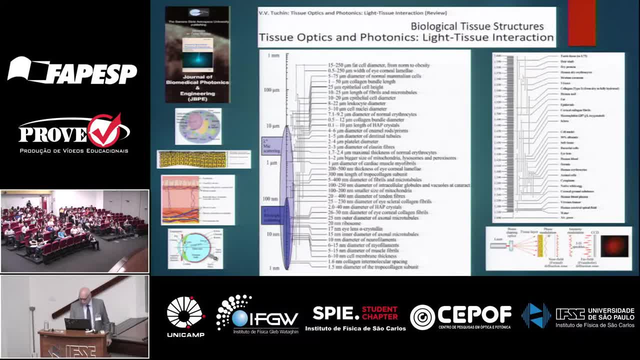 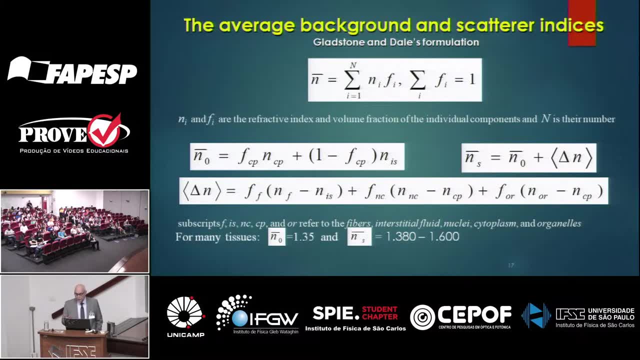 So it's very simple and very elegant approach. So, but when I talked about the origin, so this is also very nice law. probably you know about law. It's very fundamental law, Gladstone and Dali. formulation And physical background is that if you have a mixture, 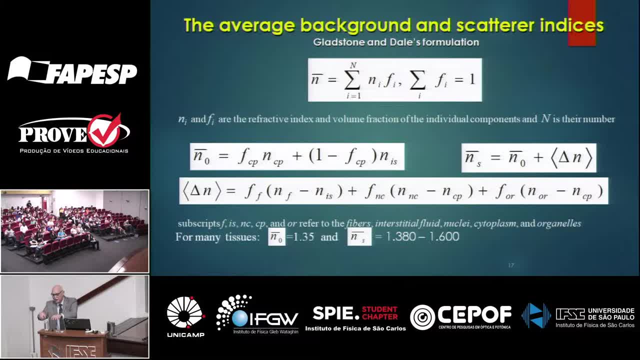 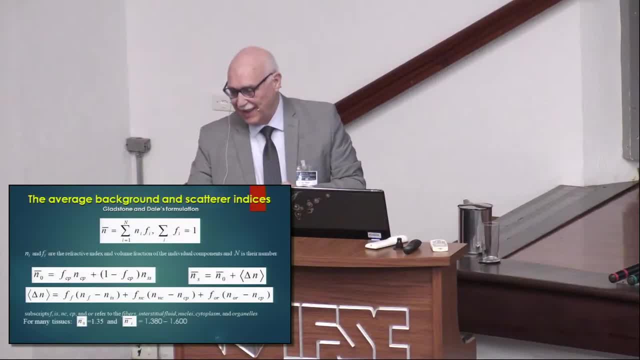 of different particles or scatterers or whatever you like, or components with different reflective indexes. here, if you're probing it by light, each part of the system is interacting independently for some, indeed, limits, And therefore you can combine them with their weights. So a lot of small particles with high reflective index. 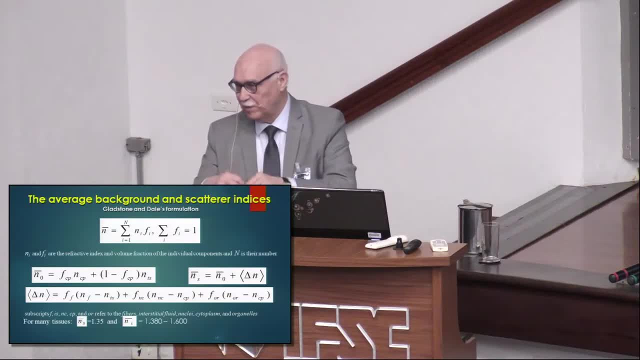 and vice versa. you have a lot of small part of the particles with the other reflective index, So you have a volume fraction, So you have a number of the particles of each And that means that light, indeed light more complicated, because first it met some small, then big, and so on. 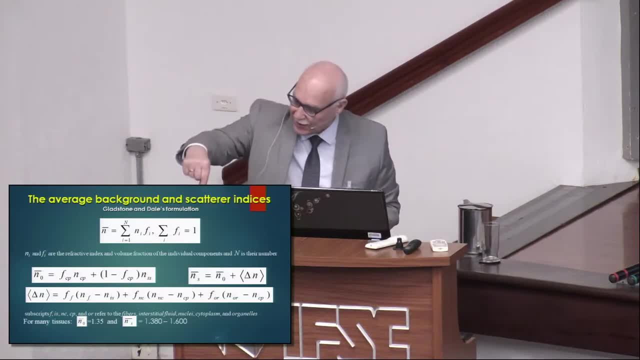 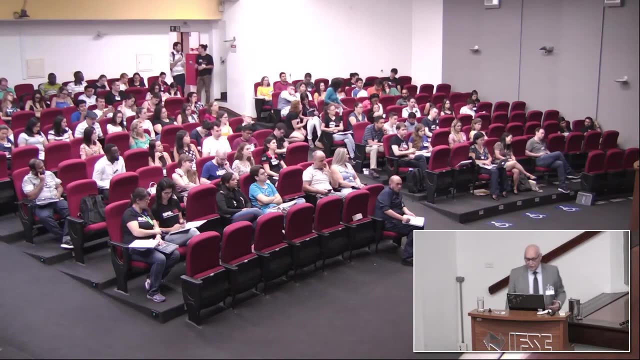 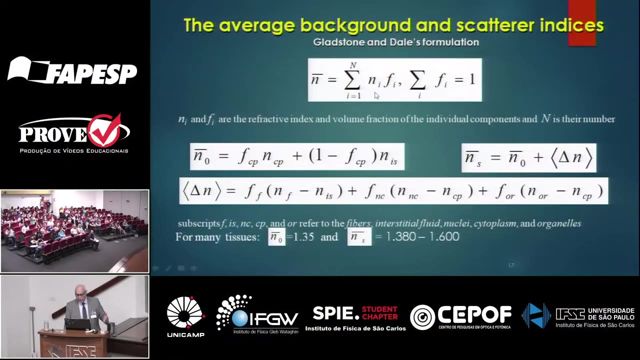 But finally the phase shift here will be the same. So if you're not interested in what has happened inside, outside, you see, you can combine them Because and in that case you have a reflective index or a delay of the light, the phase delay of the light. 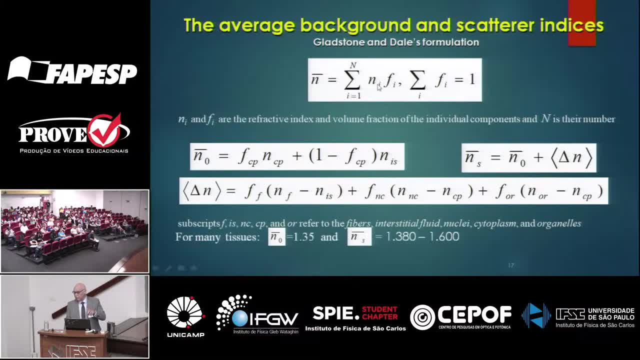 like a sum indexes of companions with their refractive fractions, their volume fractions. So indeed, it is volume fraction unity, because you can easily 80% and 20%, 60%, 40% is easy to define. So in our particular case, when we are talking about this model and we would like to calculate, 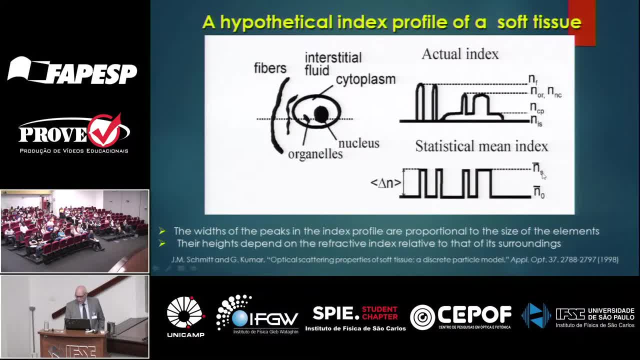 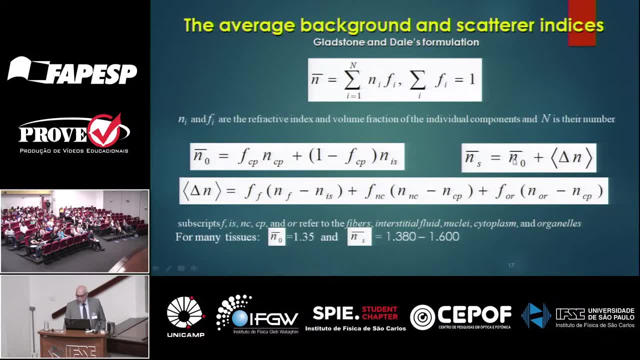 the scattering coefficient, sorry, refractive index of the scatterers and the background. we can do it for our system as this one. These are the scatterers, some refractive index of the background with the cytoplasm and interstitial space, and this some extra refractive indexes. 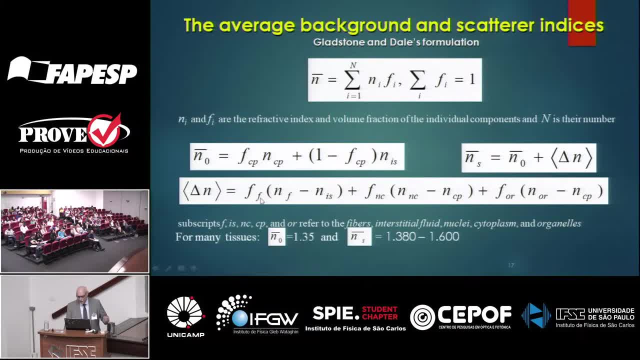 which can be calculated for the refractive indexes and volume fraction of the scattering of the fibers of the nuclear and organelles. So typical numbers is: for background is 0.1, unity 0.35, and for scatterers it is in the range that depends on the, for example, tooth 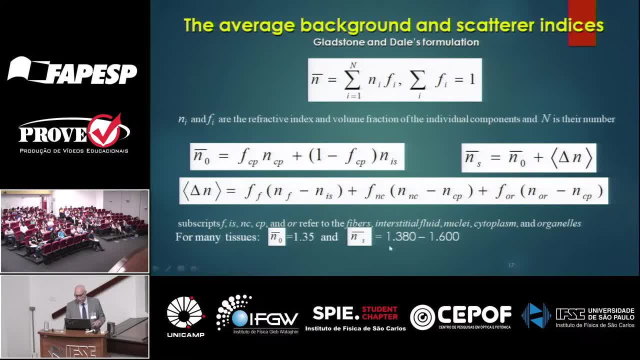 ML or some other bone and so on. So this is the range for the scatterers refractive index. Therefore, these two parameters only define the scattering coefficient and under therapy factor as well. Indeed size important for factors. factor, But only limited number of. 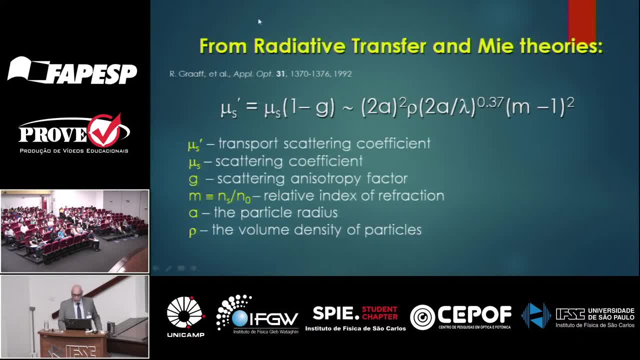 parameters is responsible for that. Also, maybe a bit earlier, because I will talk about radiation transfer theory later on. I will talk about the transfer theory later on. I would like to present the formula which I received by Graf many years ago And he did very straightforward modeling. 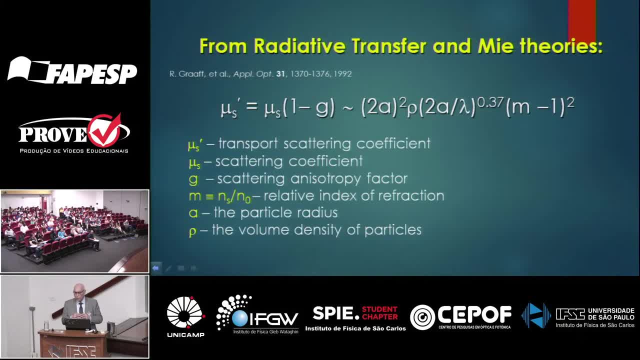 He took radiative transfer theory and tried to solve it numerically using the Monte Carlo simulation. Indeed, he used as a phase function Mi theory. After that, by fitting in the limits typical for the limits of parameters or range of parameters which are typical for tissues. 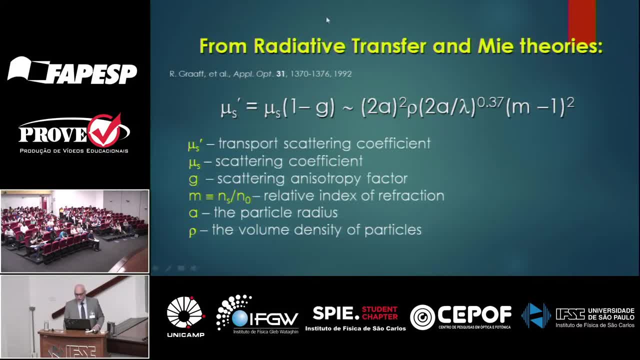 he found this formula for reduced scattering coefficient, which is equal to scattering coefficient which is reduced or corrected by this construction, where G is the scattering anisotropy factor. So you know that scattering anisotropy factor for tissues is approximately 0.9.. 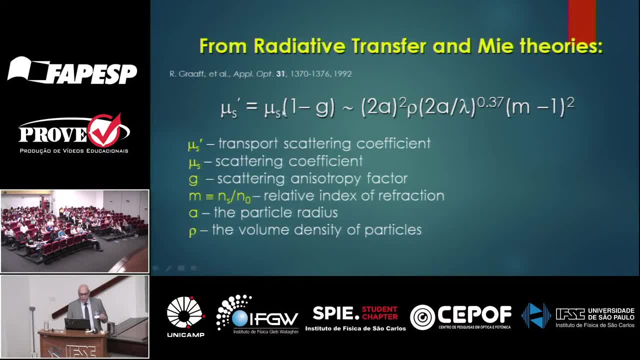 So that means that if you have some scattering coefficient which you can use in the single scattering law of Buger's law, you have to correct it 10 times, So 10 times smaller than the real scattering coefficient. Why? Because we have scattering, only forward scattering. 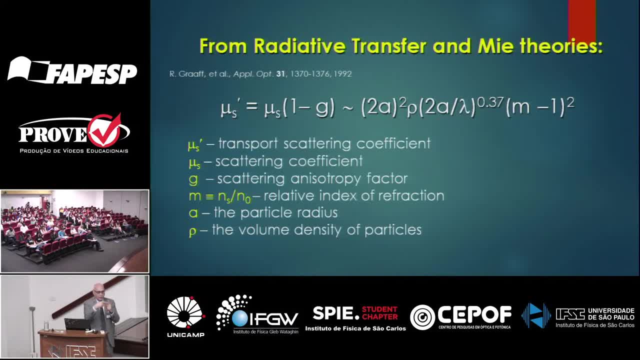 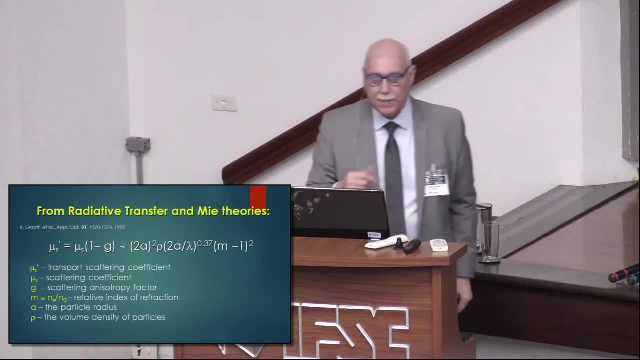 And you have some steps for photon to go from the forward direction. So these approximately 10 steps for this particular tissue. But for us now it's very important that we have a formula, a simple formula for estimation that reduced scattering coefficient indeed depends on the diameters of the scatterers. 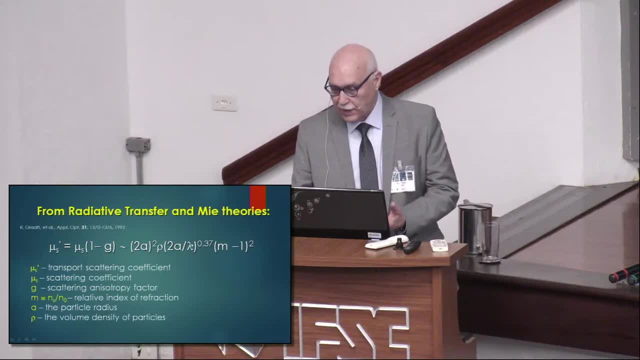 density, very weak dependence of the wavelength, And for us it's very important this ratio, or relative reflective index, or the ratio of the reflective index of the scatterers and the background, And it is squared. That means that scattering coefficient and reduced scattering coefficient. 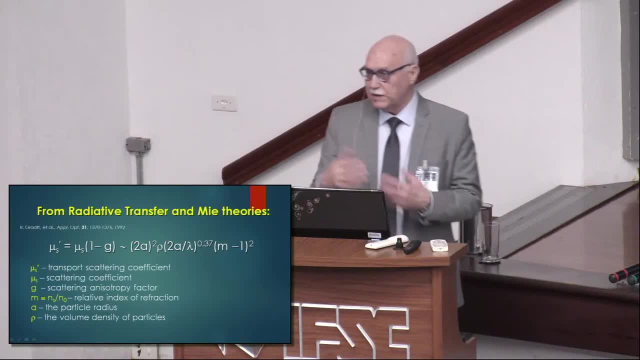 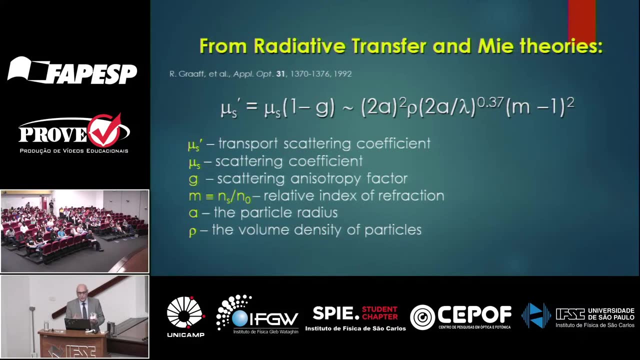 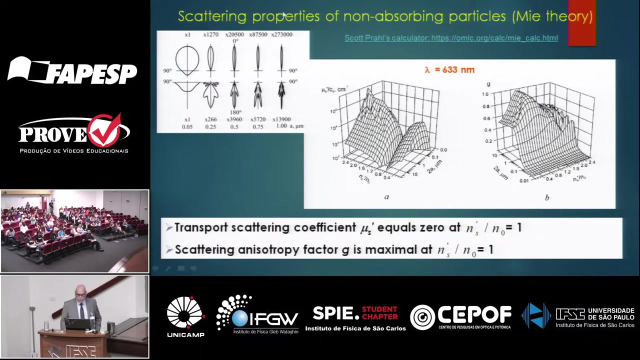 are very sensitive to the reflective index mismatch. This is the way to go to the or to design the technology of optical clearing. So you have to change this parameter and it will be very, very responsive. So to see how the It's also well known. 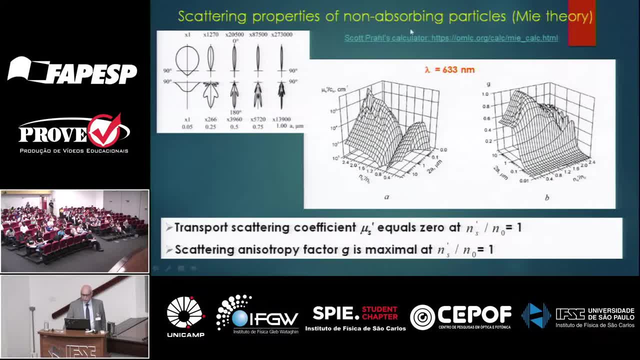 Let's talk about scattering properties. I would like to remind you this is not absorbing particles. This is me theory, And you can find some calculator on this website of Scott Prowl And calculate. this indicatorizes for your particular system. So indeed, this is. 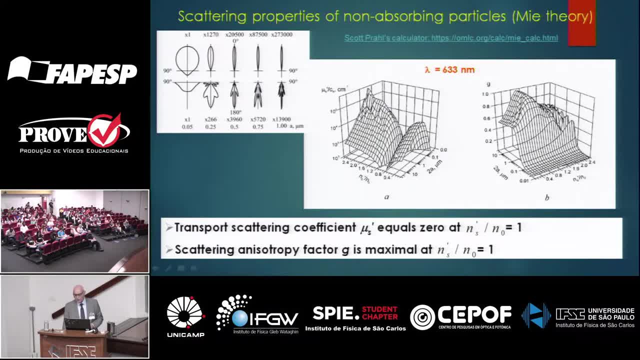 It is not done from this calculator. This is done by Professor Mueller's group from Berlin, And this is showing us how the reduced scattering coefficient depends on the reflective index. mismatch depends on the diameters of the scatterers and how the anisotropy factor 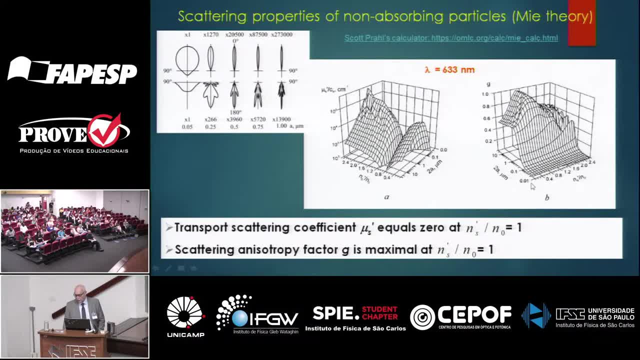 depends on the diameters of the scatterers and the reflective index mismatch. The most important for us here that indeed it's evident. when the reflective index mismatch is zero, so unity, they are matched. then M equal to unity, we have no scattering at all. 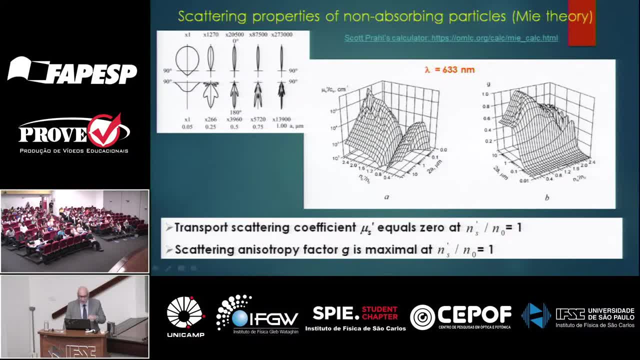 But another point, very important, also used in biology very often, in particular for gold nanoparticles, for example, or for some bubbles within the blood. So you see here also, indeed, this is inverse ratio, So that means that we have some bubbles. 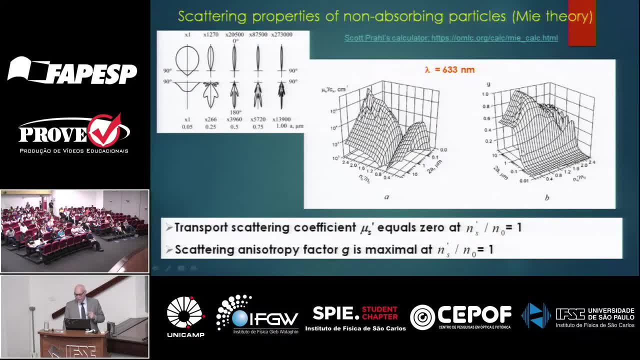 This is for bubbles, this is for tissue. And another important thing that you can see that for reflective index matching for rather big particles, we have Z factor equal to unity, Very, very anisotropic, scattering, Very, very, for example, 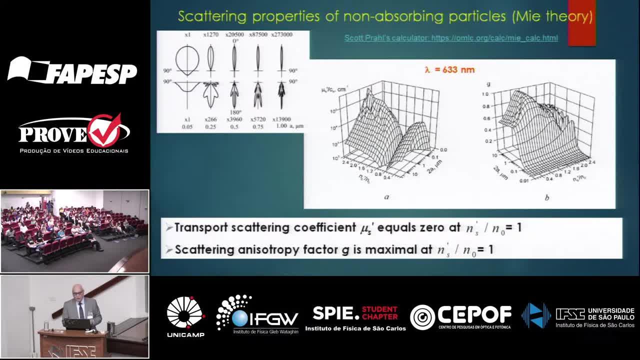 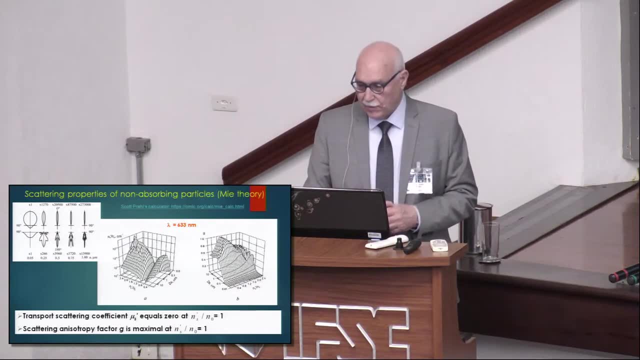 like for blood, And that means that we can use some interference effects to measure, and so on. Also, this is some basic for optical clearing as well. Indeed, it's easy to get, It's evident, but we have to provide it in technology. 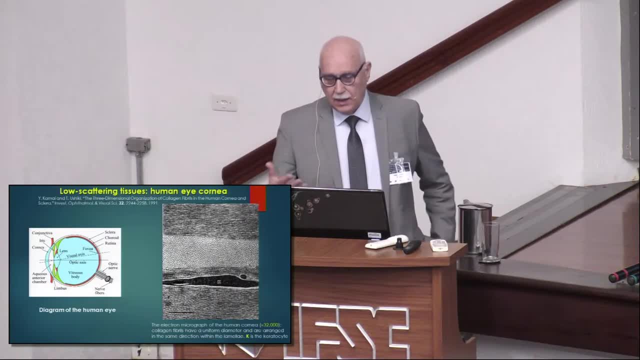 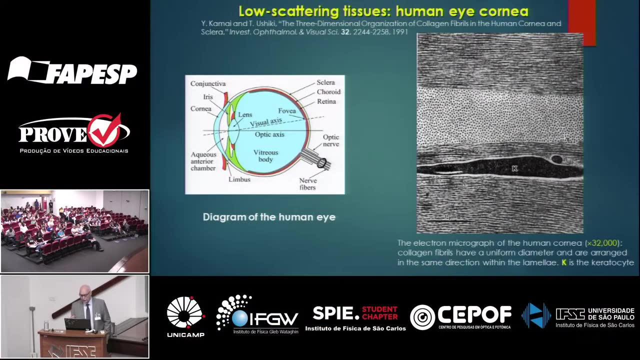 So once again, let's go back to low scattering tissue, because this is a good example to understand what has happened during the clearing process. So this is once again human eye, this one, And you see here very interesting structure. This is quasicrystal, as I already showed you. 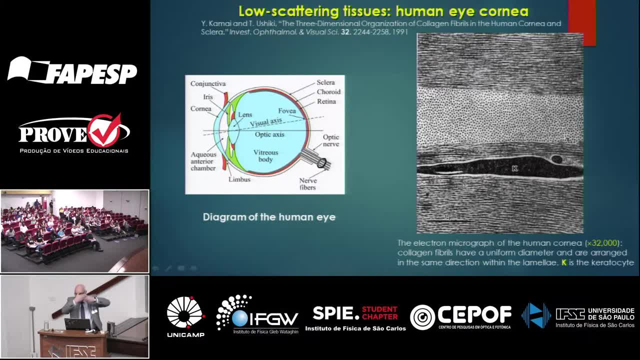 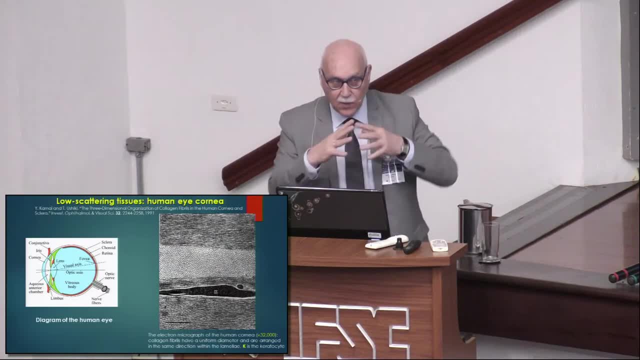 And we have some lamellas like a bandage here, here in this direction, collagen fibers And therefore the cornea is the lens- good lens- And it's thicker in the central part and thinner when it's connected with this- clearer. 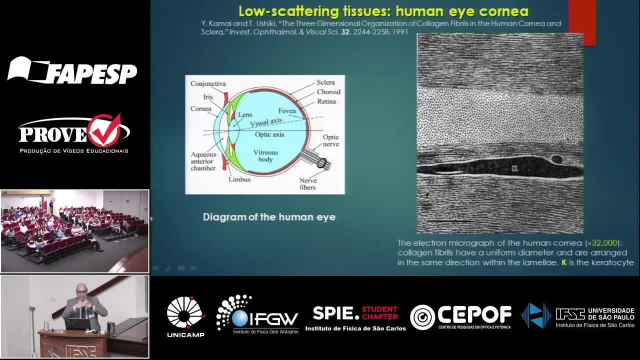 you see here this one. So it's many, many, many lamellas- about 300 lamellas, And within each lamella this is lamella. you see, here we have a very nice structure. Let's go a bit here. 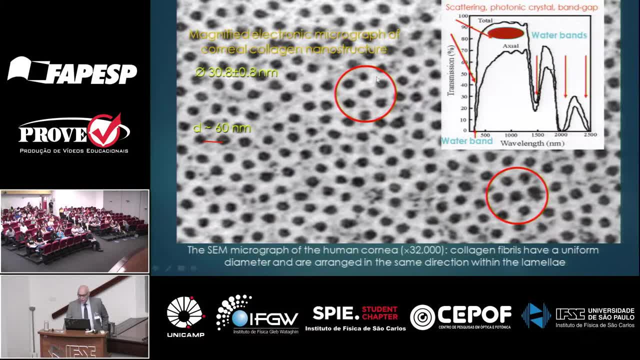 because I'm talking about cornea. This is quasicrystal. you see here, here is an all form of quasicrystal. So you see, this is nanostructure, this is matte material done by nature. because you see here, 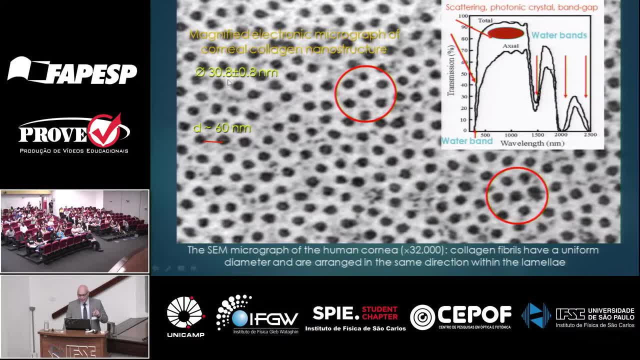 diameter 30.8 plus minus 0.8 nanometers. And the distances is also very, very good, coordinated with high precision. Only this is way to have some transparency. But another point: this correlation spatial is only for local, only for this one. 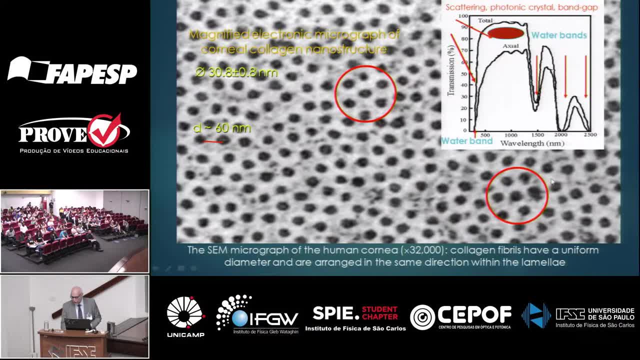 And the correlation, this one you see here or here, but not this particle and this particle. That means that we have something which are correlated very closely, give some interference and transparency, but is working for the wide wavelength range. Otherwise we will have only one wavelength. 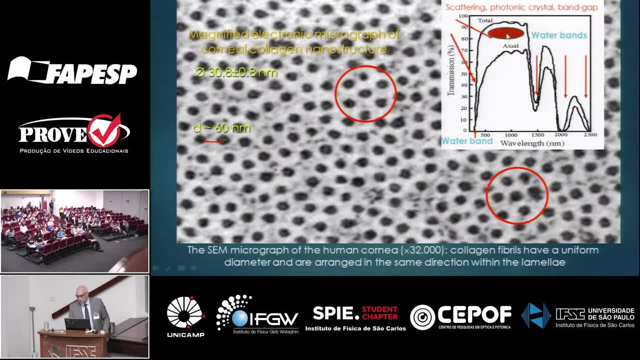 for vision. And you see, here this is the spectra of the transmittance: total with scattering and axial with no scattering. So we can measure. this is real measurements for real patient. And you see, here we have a 20% about scattering. 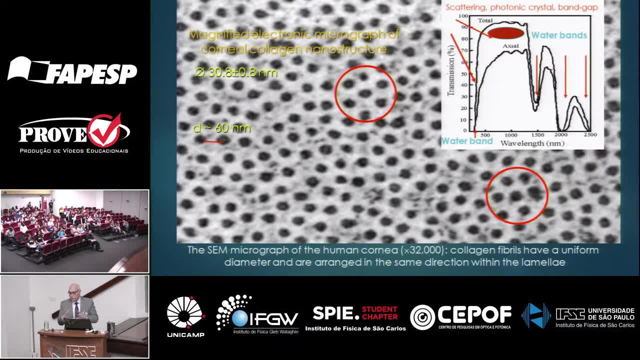 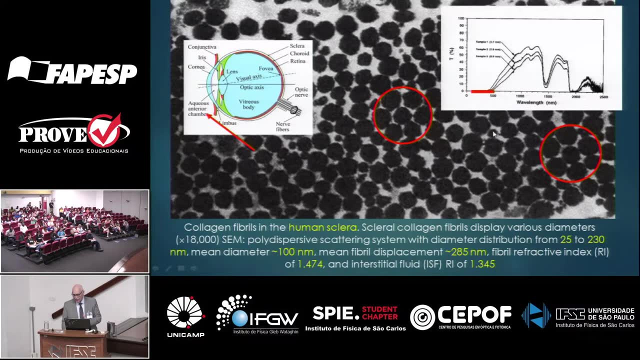 inside the eye. So therefore, scattering is really there and not totally compensated. So let's go back to sclera, Sclera, more white media, non-transparent media, But still locally we have some correlation, But it is not the. 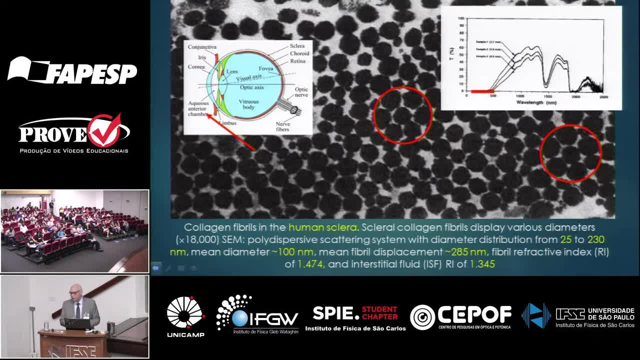 maybe play leading role here, because we have polydispersity from 25 to 20, to 230 nanometers, differences of the scatterers with mid mean diameter about 100 nanometers, And you see here refractive index for both collagen fiber. 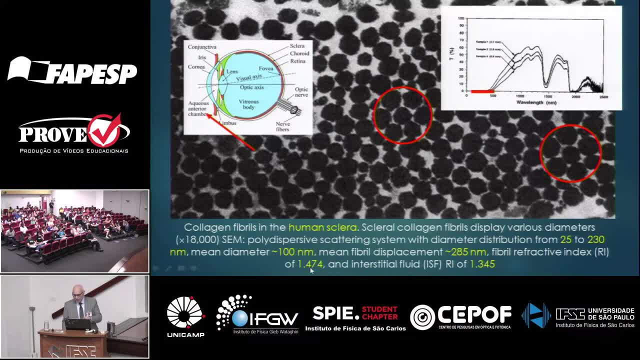 for cornea and for sclera is very high, 1.474.. And the surrounding media only 1.345.. You can calculate this scattering. Scattering is high but it's compensated because it's correlated, it's coordinated. So this is very important for us. 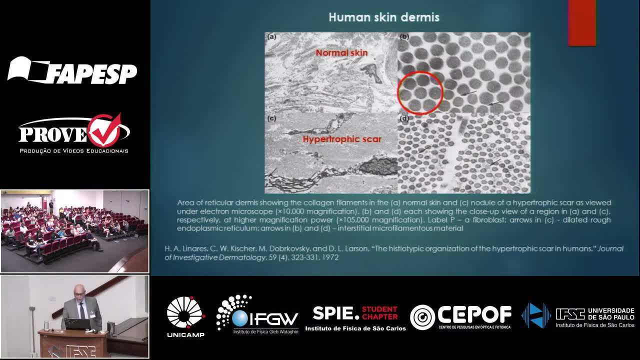 Also you can find in the human skin. It's also, but indeed the very scattering, stratum corneum. but downstairs, under this scattering, you have some ordering, And these orders can be different for normal skin and for hypertrophic scars. 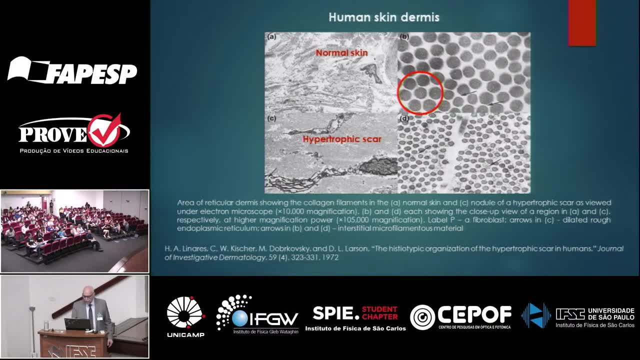 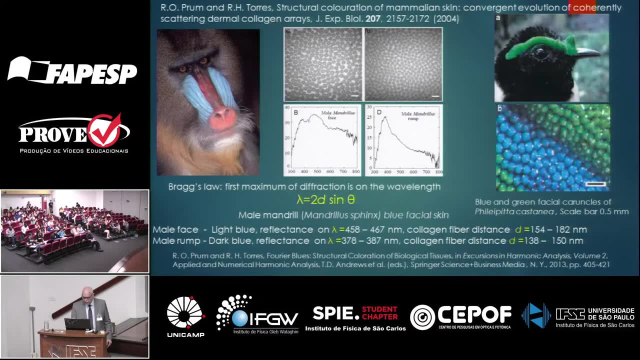 and something else Also good opportunity for diagnostics and to be have to be taken into account for some models. So also illustration, only to show you that if we have very narrow band of this diffraction on this system, you will see color immediately. 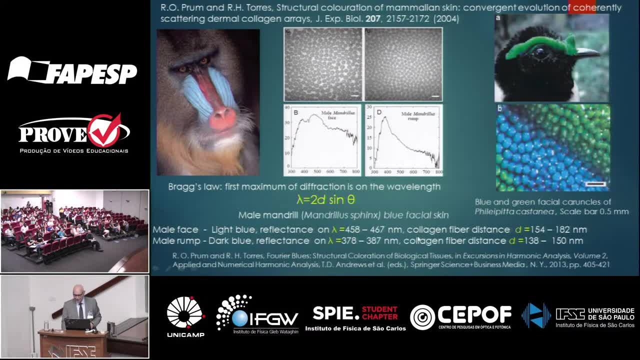 See color, color, color color. So in that case this is the same physics, because it's like a volumetric diffraction, grating, And therefore, if it is ideal, only wavelength or some, If it is more or less. 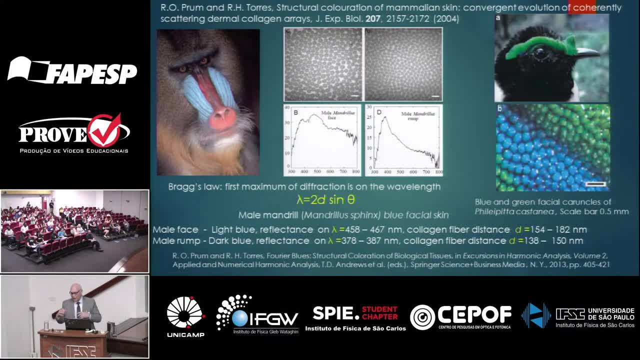 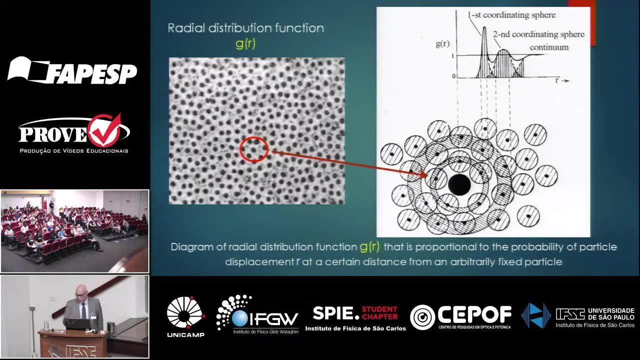 with some arrows, with some de-correlation on the big distances. in that case it's more wider and we see something. So it can be described in the framework of the so-called radial distribution function. It's another, but it's history. 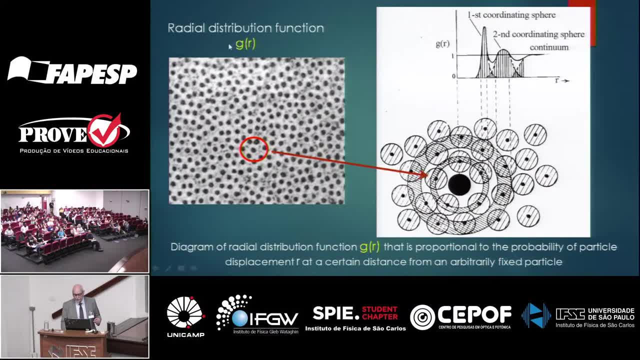 Therefore I left this nomination here from the R. If I put some particle here, other particles will be around due to some interaction, electrical interaction between these molecules and so on. Not big, not small distance, not big distance and some some probability. 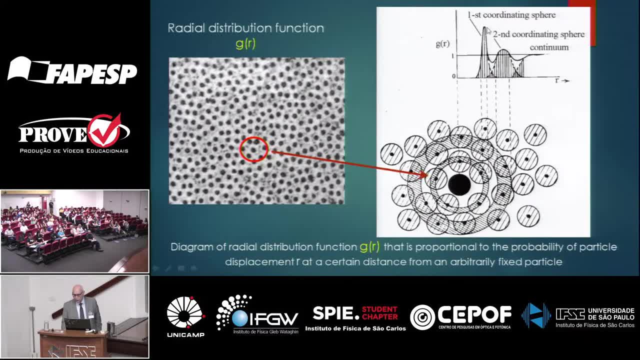 to be here. So this is the probability of particles to be in this, in this distance. So correlation, de-correlation, because it's free of particles, You can see here, free of particles layer. Then once again some correlation. 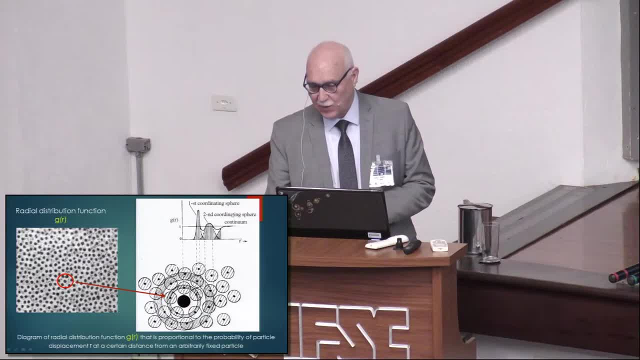 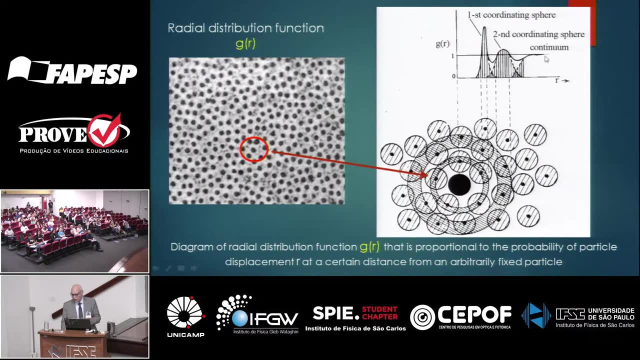 but much weaker and only two or three oscillations of this function is give you the de-correlation, fully de-correlated system. Therefore this system is more wider than the transparency for light. So you can easily if you have electronic. 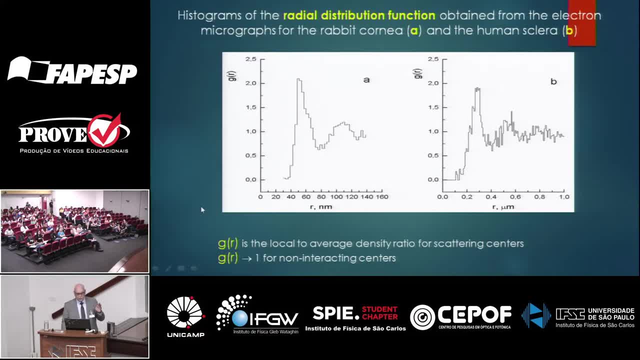 micrographs, you can easily calculate this g factor- sorry, g- at r function, estimating the number of particles around the particular particle, if you have electronic micrograph. So it was done by a group from USA, from a group of Farrell, and this done 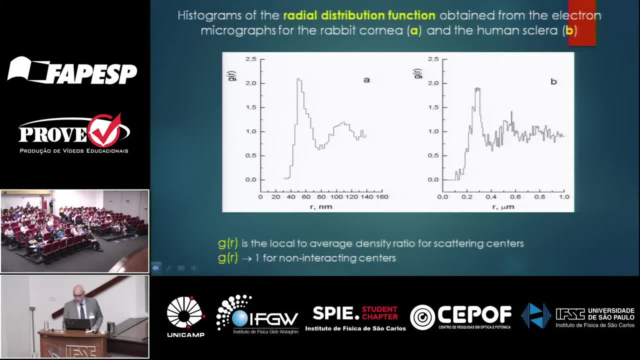 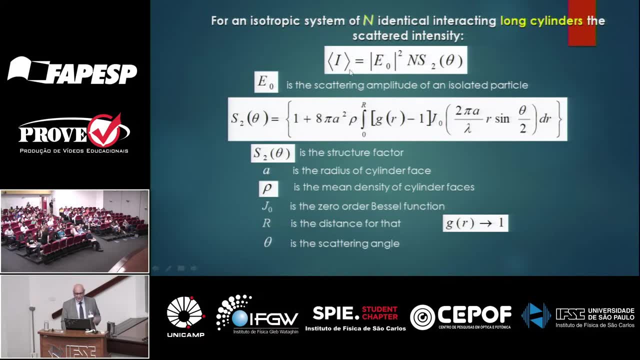 by our students for Sclera Also. we have some correlation there, So it's easy to do So. and how to account for? So probably you know this formula well: Intensity. this is the formula you see. 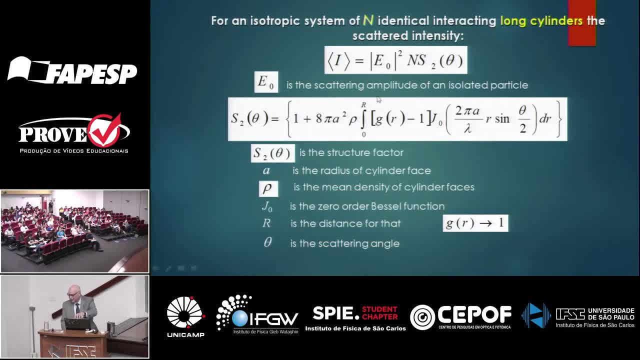 here. Indeed, you have to multiply all the number of the particles which are shining, And these are the form factor which are accounting for interference, which I'm talking about. So, which is the formula you see here? This is the form factor can be. 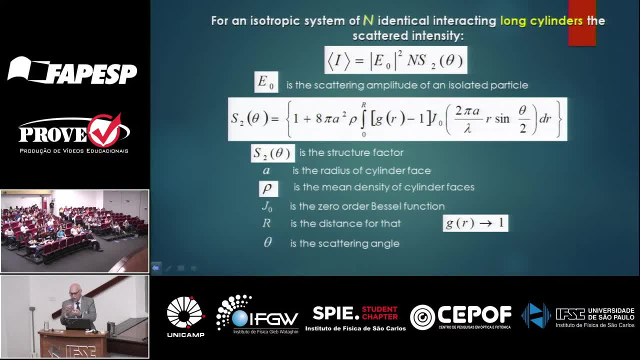 different for different for cylinders, for for slits, as you have for slits for cylinders or for for balls, scattering balls. So in particular for the long cylinders like Koerner or Sclera you have this form of form factor, you see here. 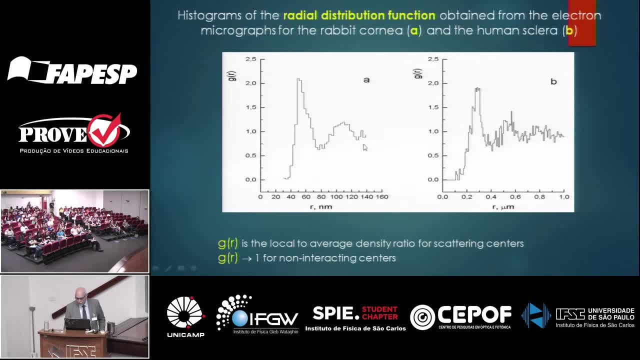 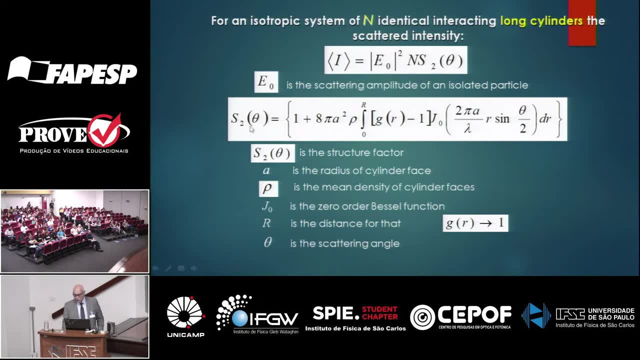 No correlation, no correlation, no correlation. it's too far In this case. you see also, zero is unity and they are randomly summarized. no interference. So we only sum scattering amplitudes or intensities of each number of particles. So 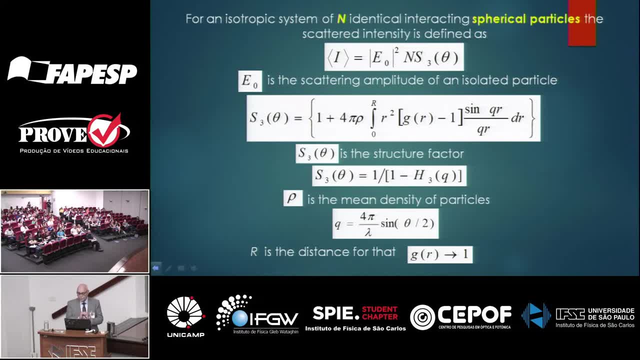 the same formula for the round, or spheres for the spheres. So I have to leave a few minutes for discussion, or, yeah, or I can finish and I will wait for tomorrow, probably. Yeah, Agree, Yeah, good, So, and I think it. 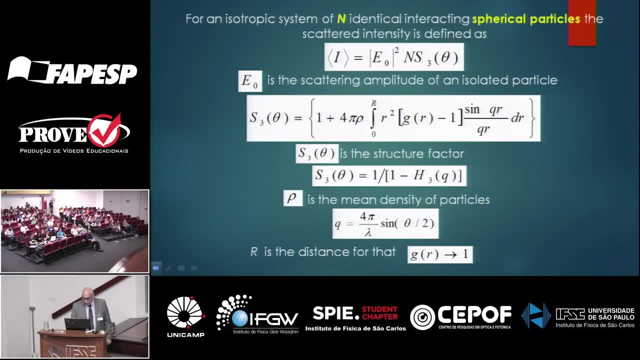 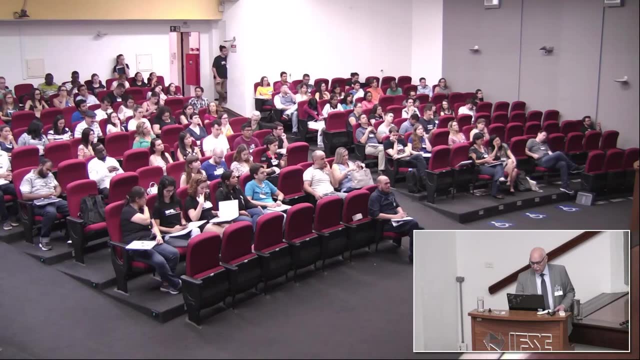 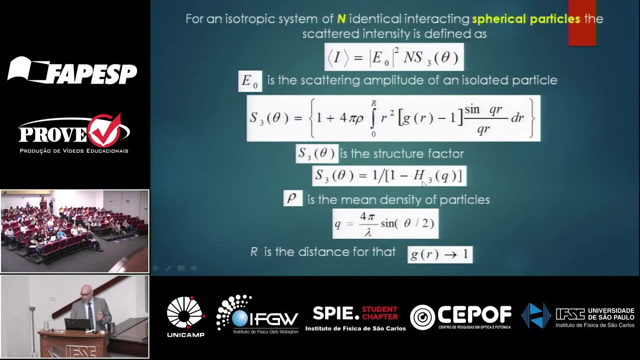 could be available for students already. Yeah, yeah, it's good. So once again, we see here another kind of form factor Indeed. it is very long theory and you can use this derivation of this equation, but it is dependent only on. 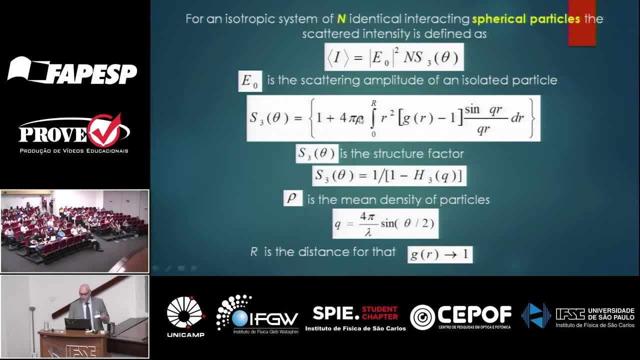 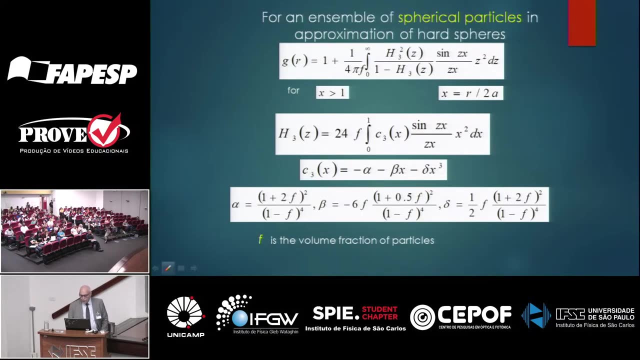 this on the, on a small number of parameters. You need only the density of your particles, you need diameters of the particles. So if for spherical particles, if we go, go, go go, we see that it depends only on the. 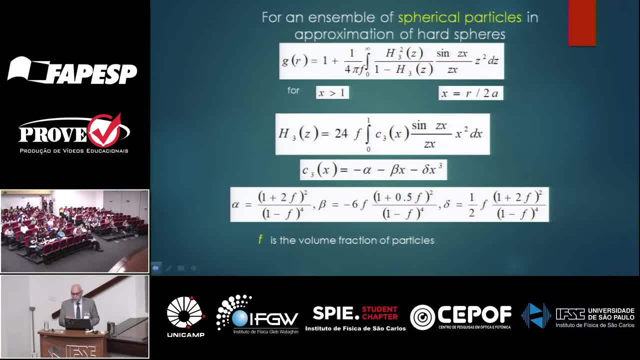 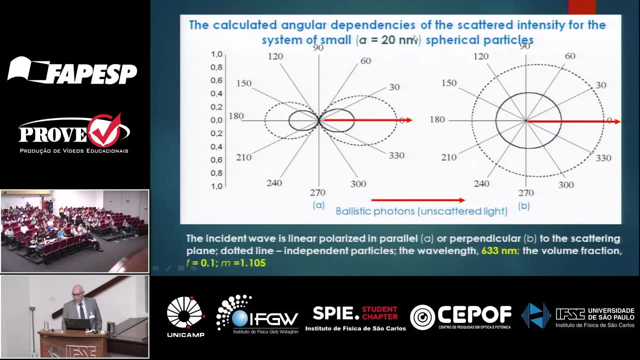 volume fraction of the particles. Indeed, you have to have the diameter, refractive index, and so on. So this is examples of the calculations for the small particles. it's nanoparticles, but it is not gold. this is nanoparticles which can find. 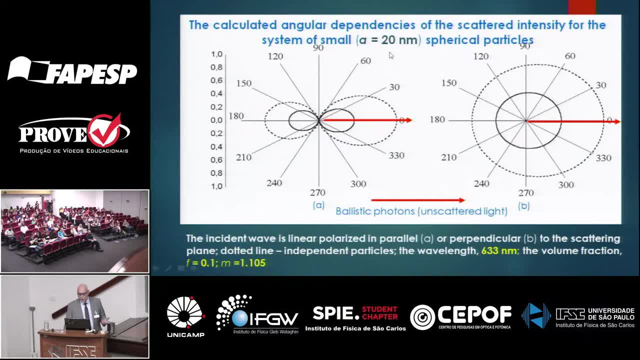 in cells, for example, some exosomes. exosomes, yes, it's in this range, also some other things. So light is incident in this direction. this is forward direction, this is backward direction. You see here, this is. 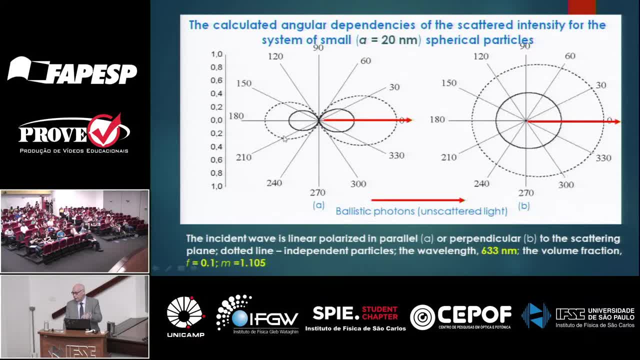 for so and two, polarization, because you know that relay- this is mostly relay scattering here and therefore any light which is incident on the system of the small particles, like relay particles. we have a good polarizer- not good, but not. 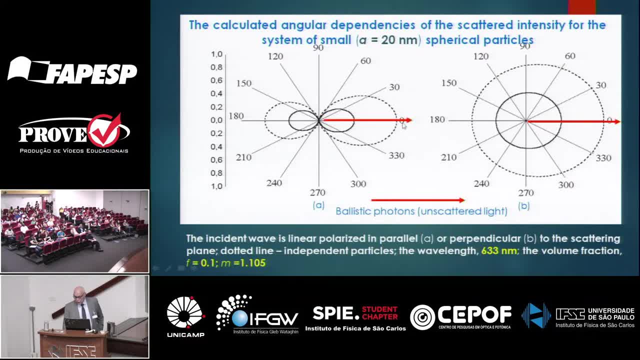 bad polarizer. So this is ballistic photons. indeed, we have some ballistic photons and this is part of scattering photons. If we have spatial correlation of the particles, we have quite limited because all light is interference and go in this direction like red. 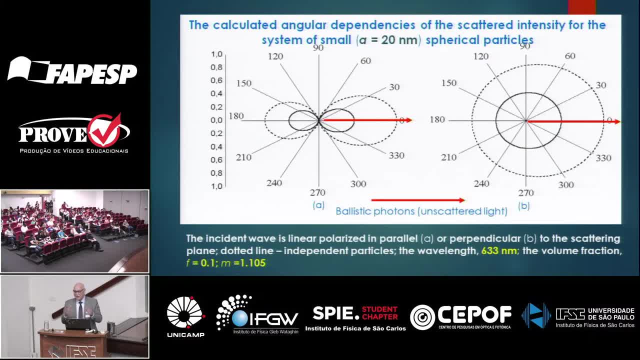 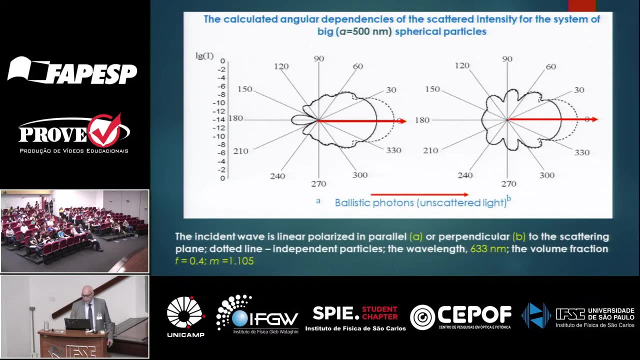 light. It added to the ballistic photons, So indeed they are scattered photons. So you know this is a big particle like 500 nanometers. You see here pretty good me indicatorizes. And you see here once again, this is: 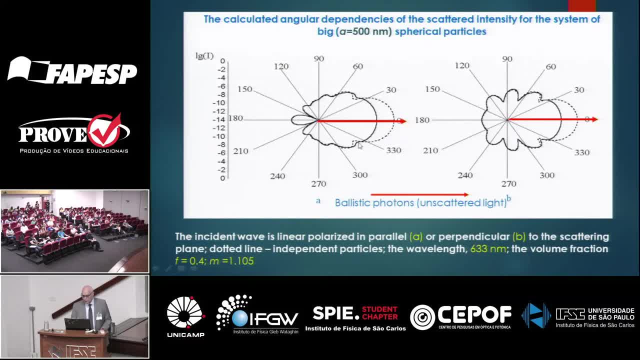 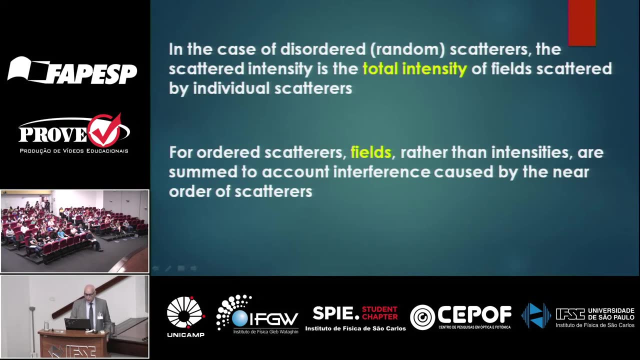 without interaction spatial and with interaction. Indeed, this is changes huge. Why? Because this is logarithmic scale here, Once again for two polarization state. So we can conclude here that in the case of disordered random scatterers, the scattered 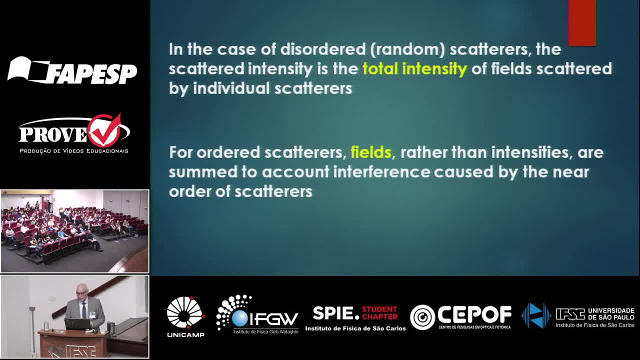 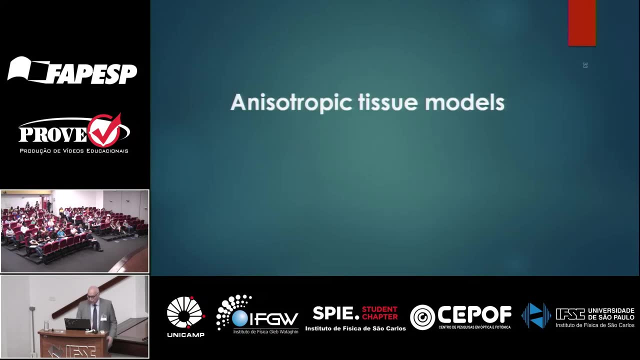 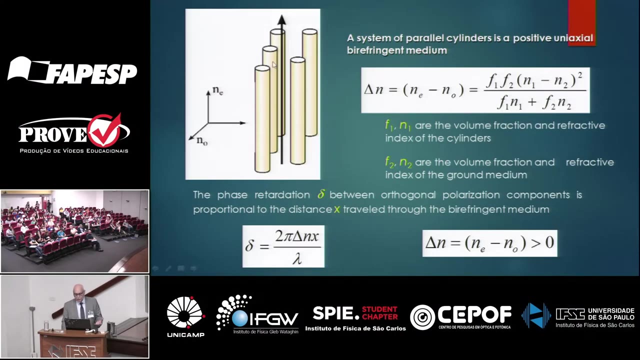 intensity is the total intensity of fields scattered by individual scatterers And for ordered scatterers, fields but not of the scatterers. So a few words about- I have two minutes, I will finish- anisotropic tissue models. So 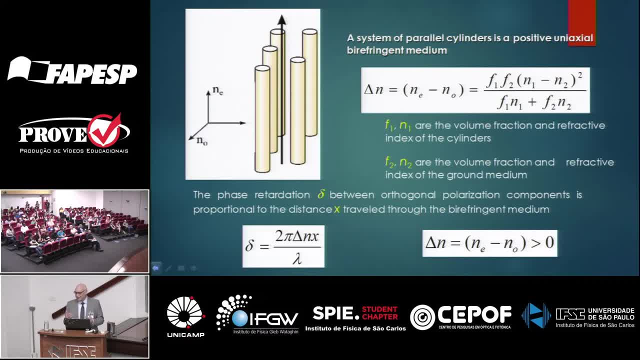 this is the cylinders which are already discussing, but because we are not talking yet about the difference of the reflective index which depends on the volume fractions of the scatterers. So this is the difference of the reflective index differences which depends on the volume. 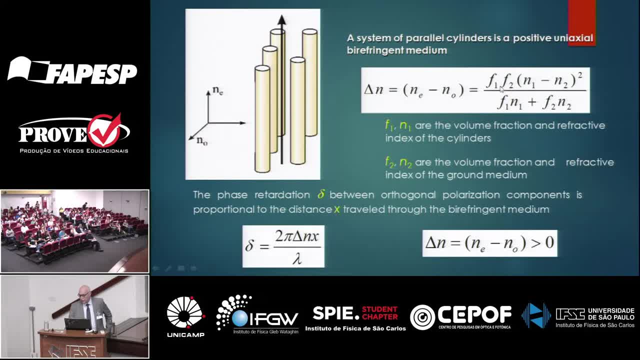 fractions of the of the scatterers With their own reflective indexes. here, Indeed, we have the same here. we have different phase shift for different now perpendicular polarized light due to specific structure, And this phase, retardant retardation can be calculated in. 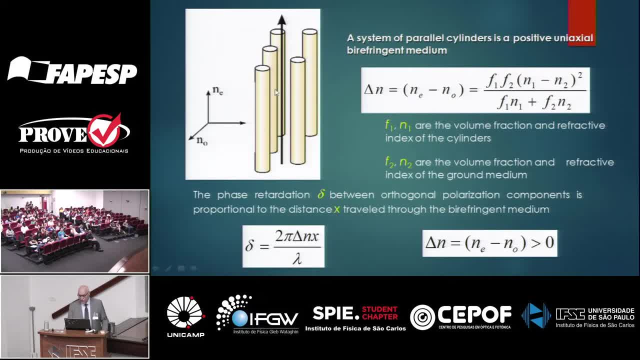 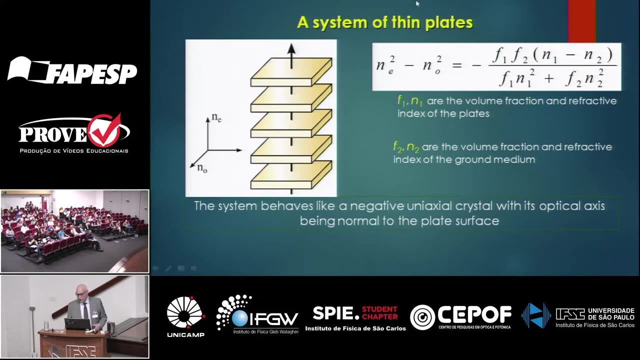 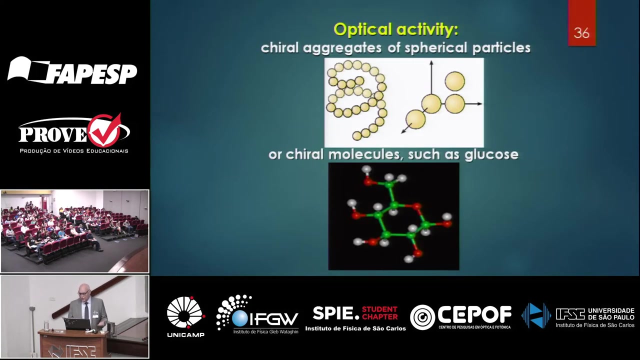 different ways. And for these cylinders, when reflective index higher than surrounding, like a model of the collagen fibers, we have this like a positive crystal with, but in that case it is negative crystal. So also optical activity. you know optical activity. 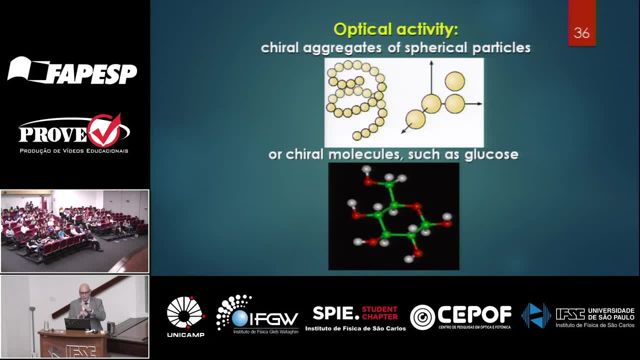 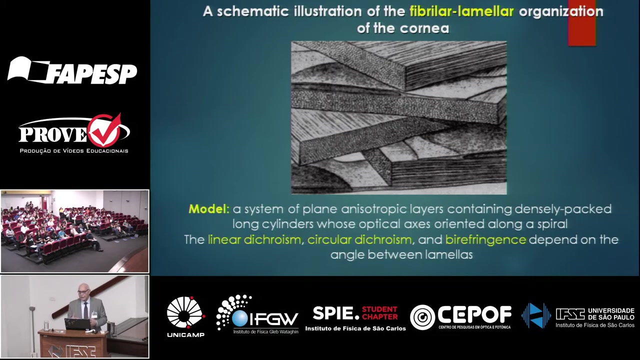 if you have some linear polarization after the system, it will be different angle of the inclination of the and like glucose, And indeed when we have a system like a cornea, we have all these all together And we have to understand what is. 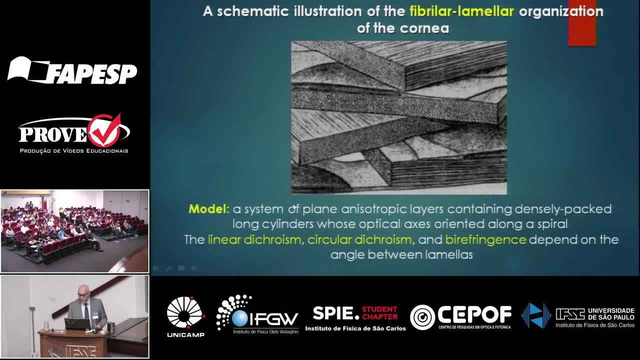 the birefringence. what is the so-called linear dichroism or circular dichroism? Why dichroism? Because we have a scattering and scattering and therefore we see it like attenuation. Even there are no absorption, So this is also. 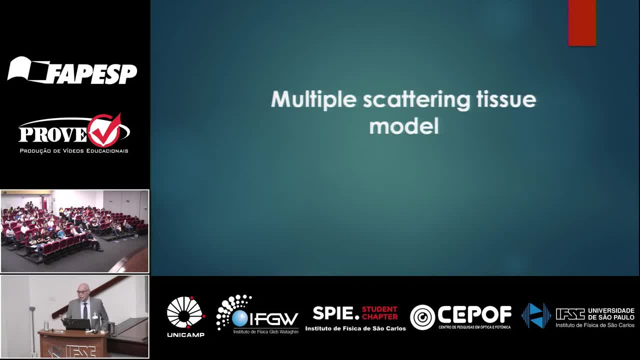 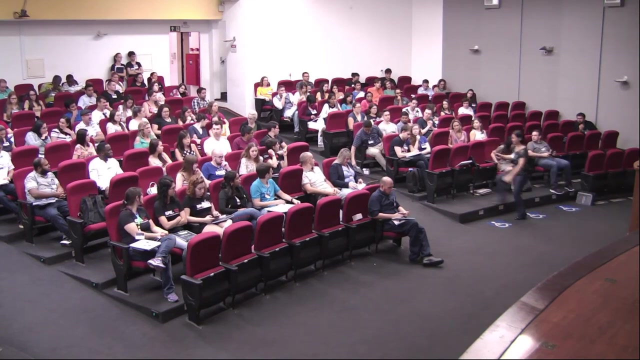 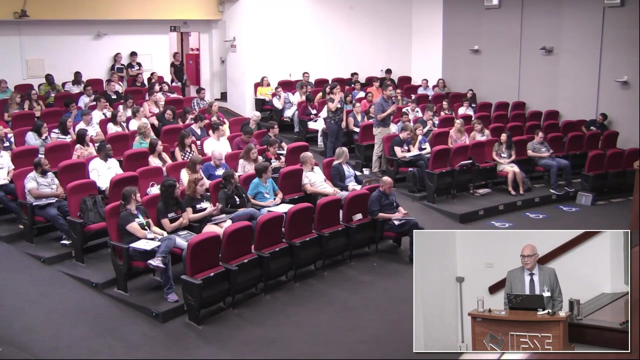 very important to take into account. So we will stop here And I'm available for questions via email or maybe here around here. Quick questions, short questions: No, No, please. Thank you for this great presentation, Doctor. My name is Gerardo. 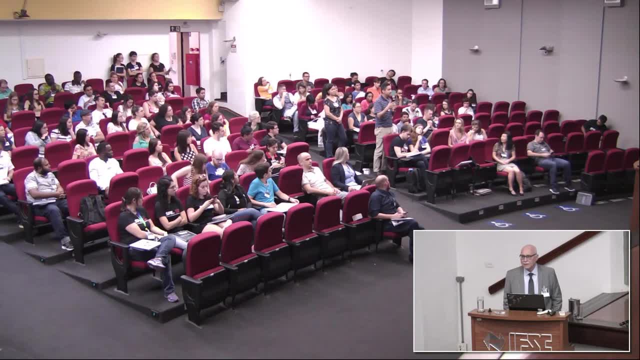 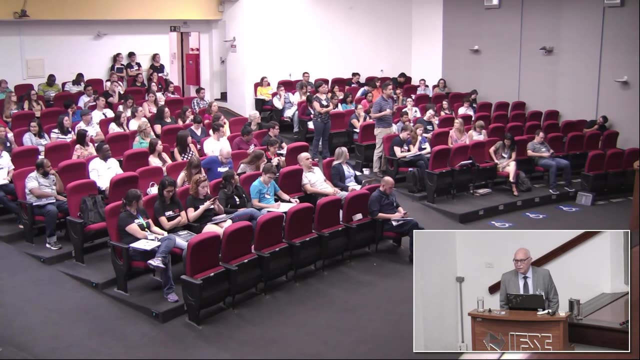 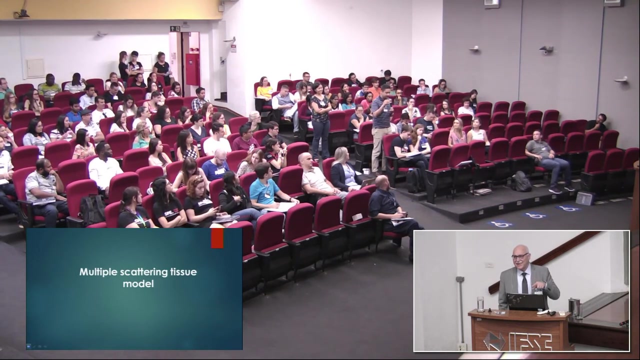 Romo from Baja California in Mexico. I have just one question, Given that the approach gives us certain limitations and thresholds for getting information back or having the light interacting with tissues. given this category, what is the best approach for getting information back or having? 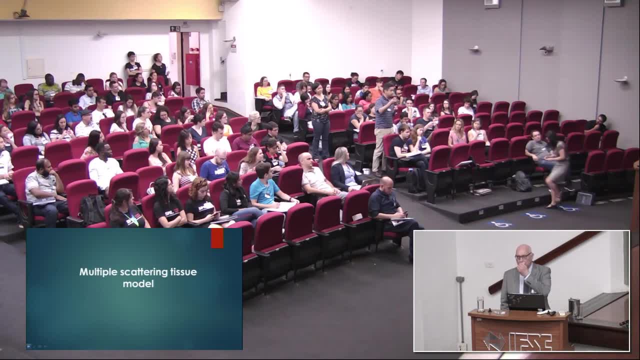 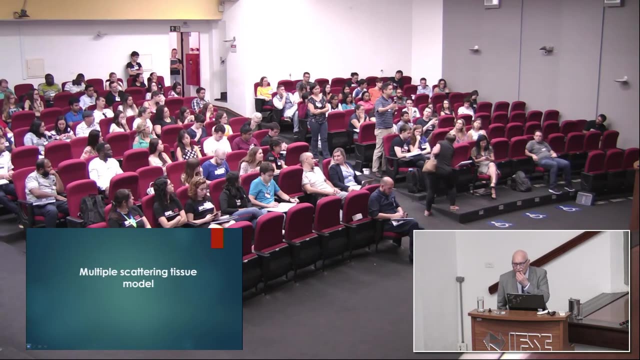 the light interacting with tissues. given the scattering and all the limitations we have in the light tissue interaction, My question is: do you think that we could use this trend of algorithms and artificial intelligence in order to explore the data that comes from this in order to pass? 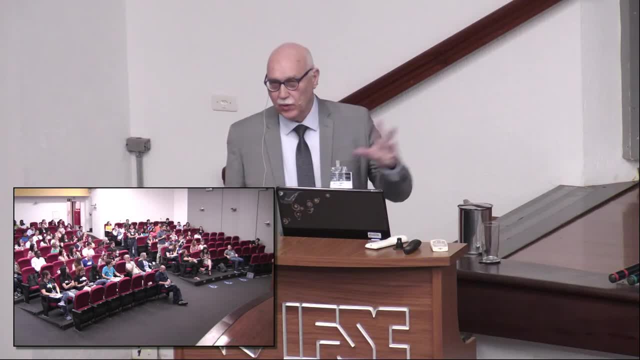 through algorithms which allows to pick up valuable information from this, maybe models or some, indeed. yes, yes, but I'm talking now only about some fundamentals. indeed, you can solve inverse of this problem with the scattering media and localize them with the high precision. as far as I know,